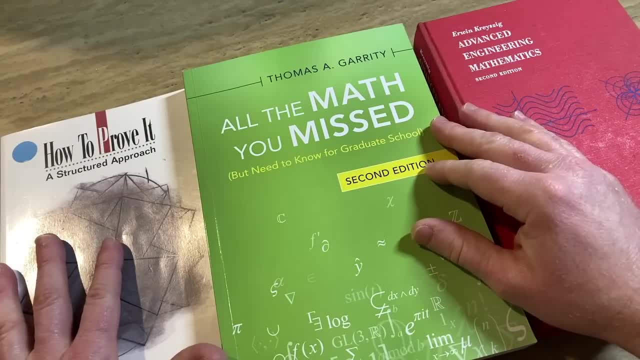 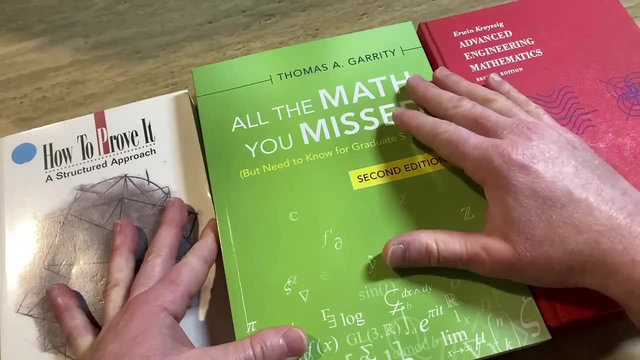 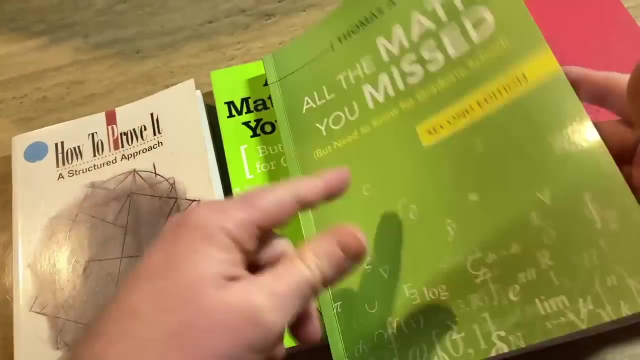 cool And they asked me if I wanted to interview Thomas Garrity, So I said yes, It was my first interview ever here on YouTube And, yeah, amazing, amazing human being, amazing mathematician, amazing teacher. This is an amazing book. So let me show you what this book is about and why it's so. 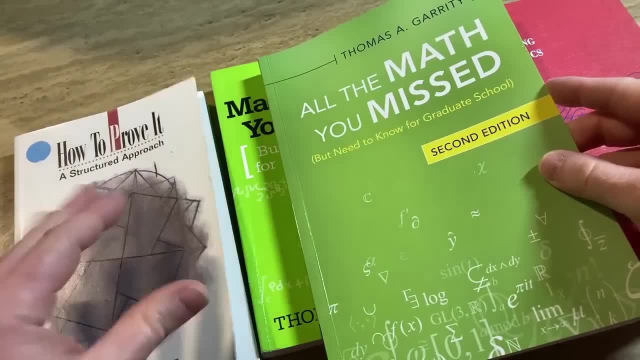 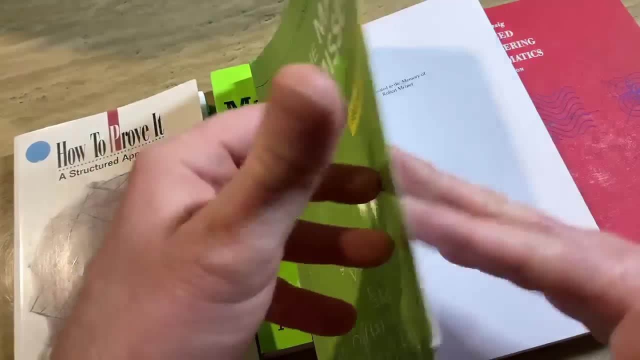 great. So it's written for students who are going to graduate school, okay, And they want to know what they need to know in order to prepare. This has more than enough information. So if you're thinking about going to grad school and you open this book and you don't know all this stuff, don't worry. 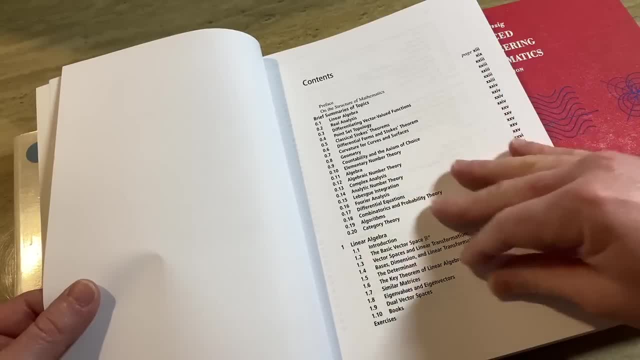 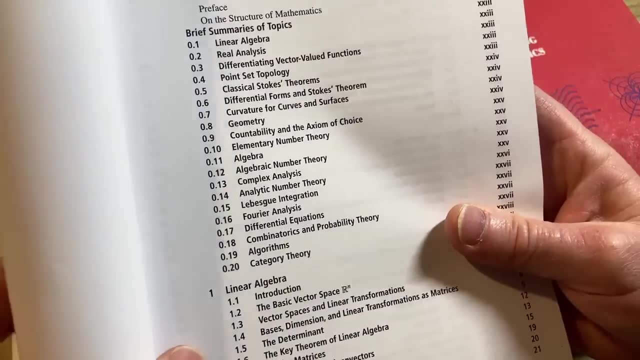 Don't feel bad, Don't feel defeated, It's normal. I did not know all of this stuff when I went to grad school. It's quite a bit of stuff. So what this book does is it gives you an overview of- I don't want to say all of mathematics, because that's not possible. 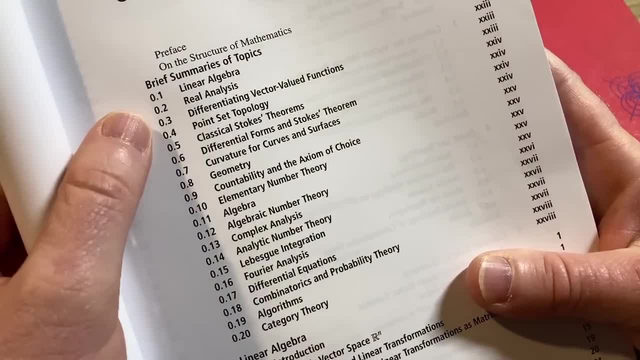 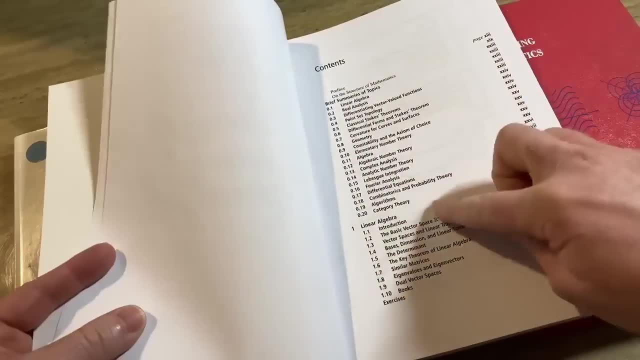 but it gives you an overview of the things that you need to know in order to prepare A lot of mathematics. So you see, it starts with linear algebra, real analysis. Look at all those topics, Tons of topics- And then you see there's little subsections for each topic. Now some 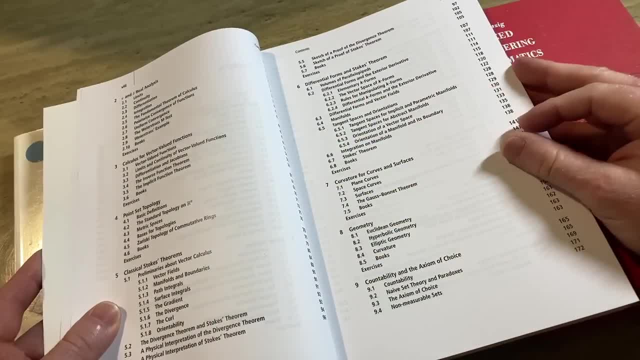 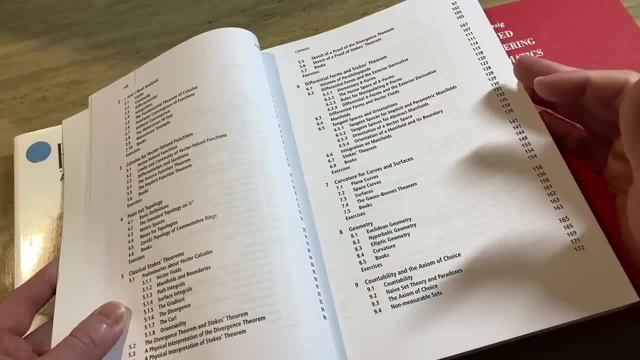 people ask: can you use this book to learn math? Sure, yeah, but you're not going to become a master at everything with just one book. It's not really possible. What this book does is it opens the door for more exploration. It really will pique your interest in mathematics. 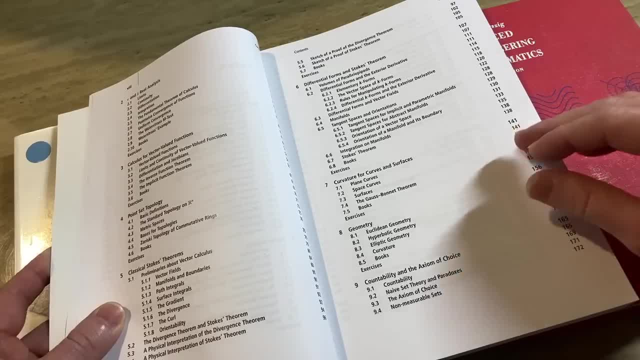 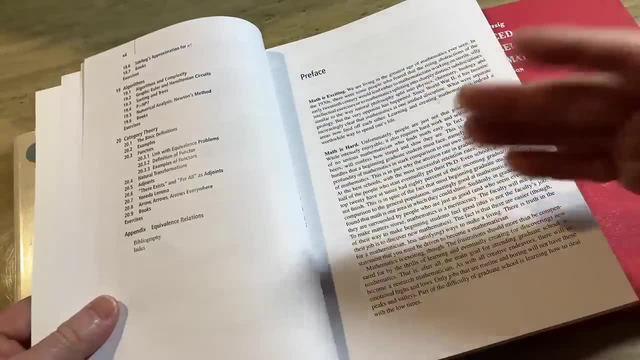 So if you're interested in mathematics and you have some mathematics background, it's worth picking up A lot of the stuff you won't understand- and I'll show you why in a minute- because you have to have some background. But if you know some math you can understand. 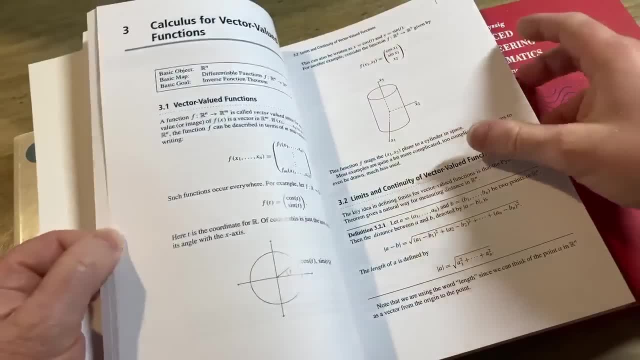 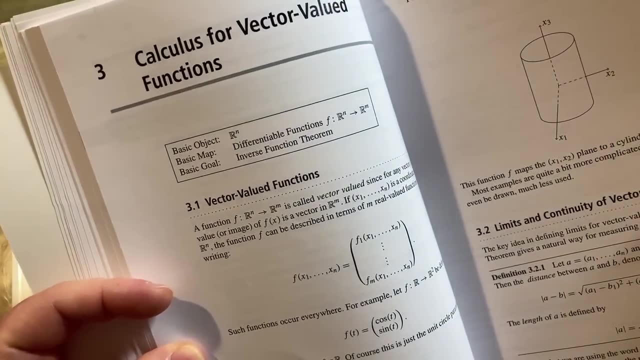 most of it. So let me just show you the main layout of the book. For example, this is three. This is really cool. Look, calculus for vector-valued functions. The basic object is Rn And then you see the basic map: differentiable functions from Rn. 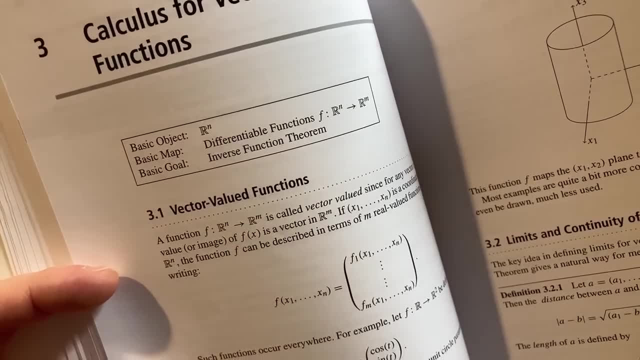 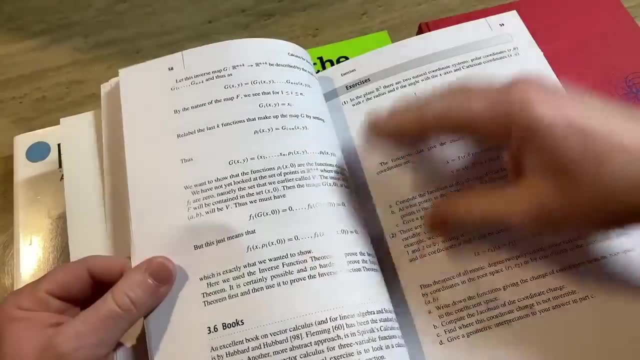 into Rm? Yep, couldn't see it. That's an M Basic goal, the inverse function theorem, And so Garrity does that throughout the book. He basically has that layout in each section, which I think is really cool. Let's look at this one. I think this is the one on topology. Yeah, point set topology. 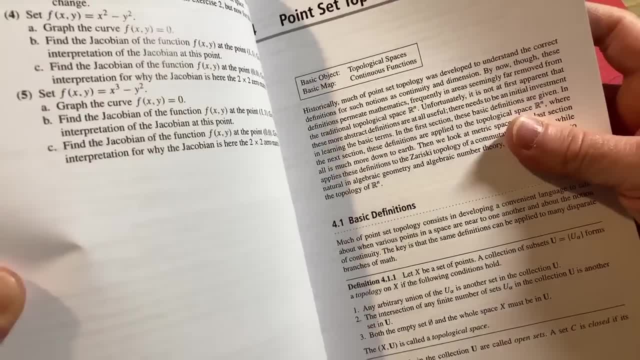 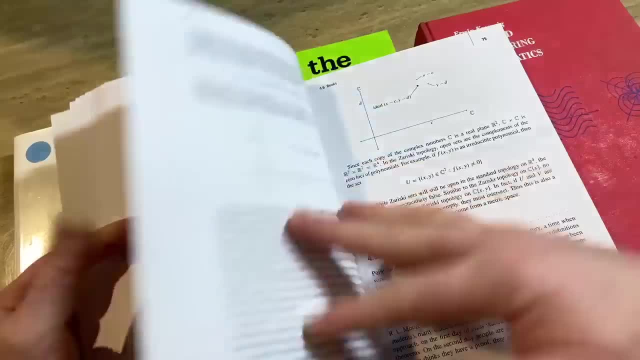 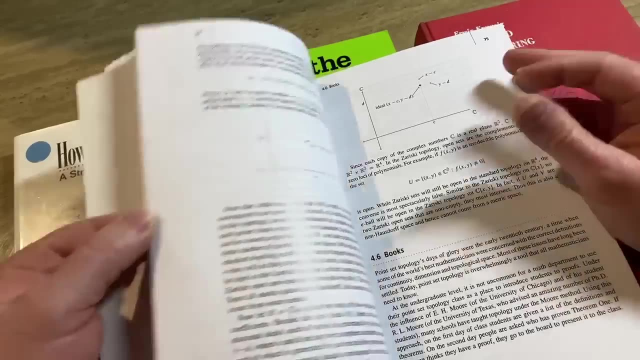 Basic map- topological spaces. Sorry, basic object: topological spaces. Basic map- continuous functions. Yeah, cool. I'm looking at my screen as I film this because this is actually projecting onto my computer. It's my live stream setup. That's why the mic sounds better, hopefully, than my regular mic, that I 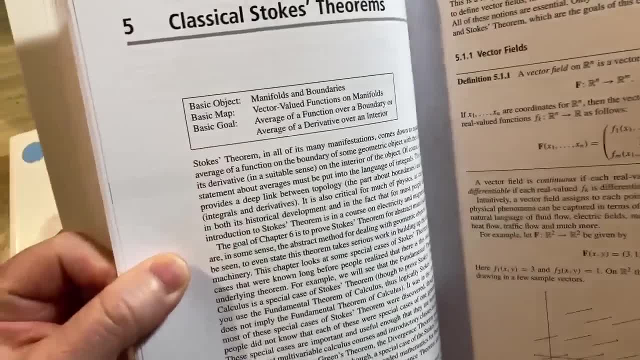 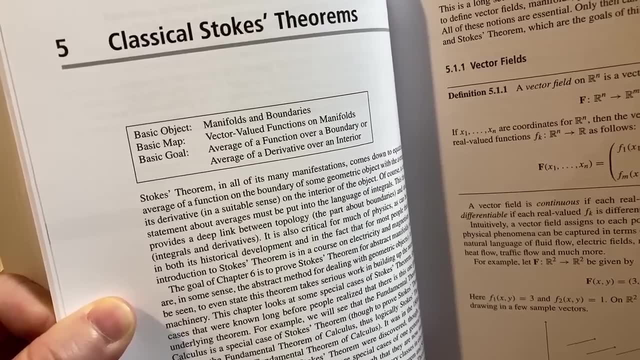 have Classical Stokes theorems. So basic object: manifolds and boundaries. Basic map: vector-valued functions on manifolds. Basic goal: average of a function over a boundary or average of a derivative over an interior. So wonderful book, I just got to give it a whiff, Just got to bring it closer to my 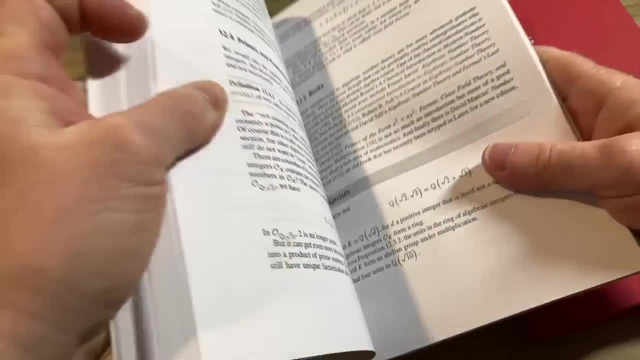 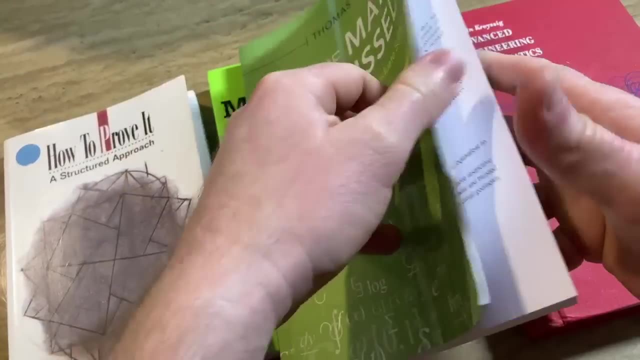 nose. Ah, wonderful book. Highly recommend it. It's heavy too, It's thick, So it's well made. They did a good job. the publishing company- I believe I should know this because they emailed me It's Cambridge University Press- Yeah, they did a really good. 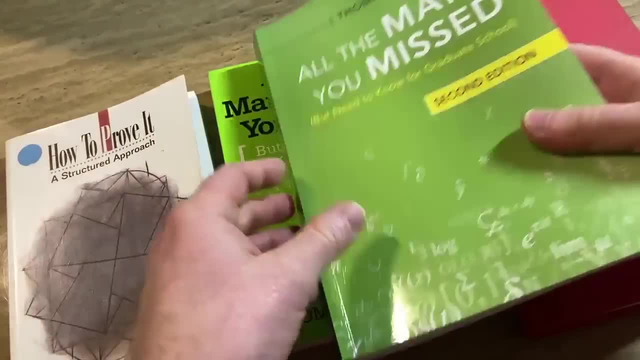 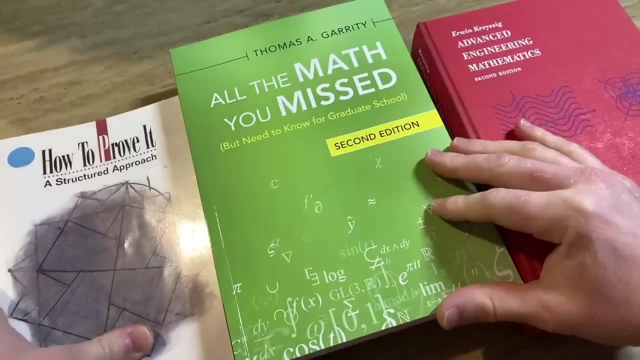 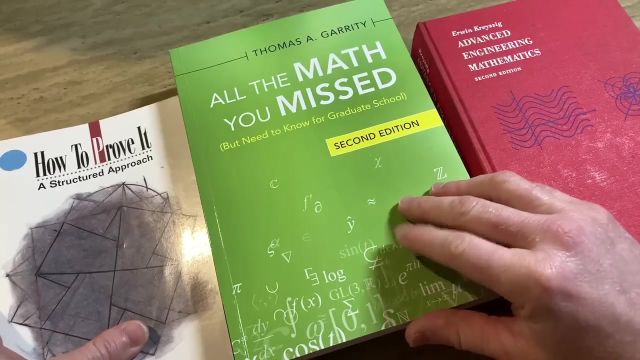 job. Even though it's a paperback, pages are good quality and like it's heavy, This is like a really heavy paperback. It just feels really well made. So good work there with the publishing. I do wish there was a hardcover. I have come to appreciate softcovers more And the reason is actually in 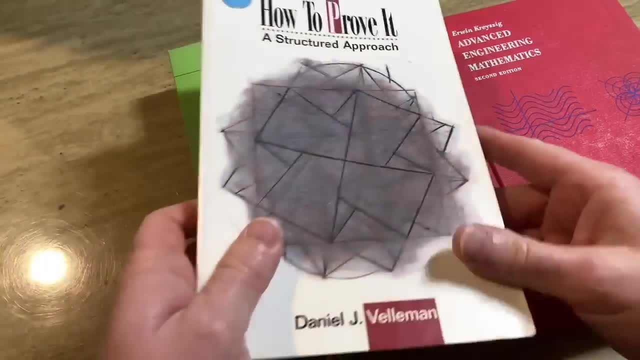 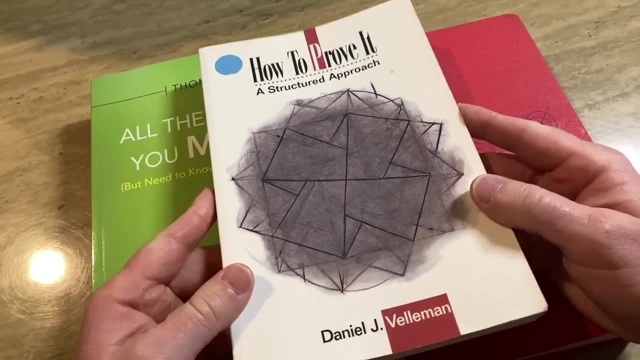 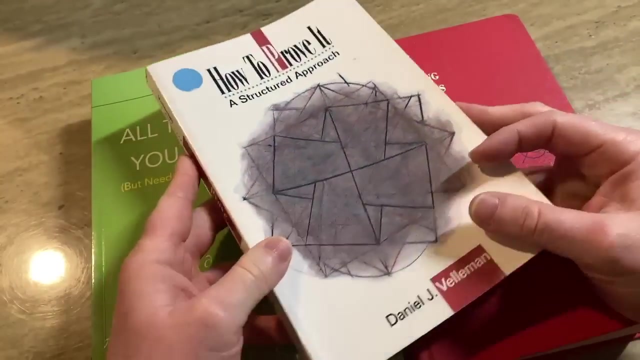 this video. It's this. This book has made me appreciate softcover books a little bit more, because this book I laid in bed and read when I first got it and I loved it. So people kept leaving comments about this book. They said: 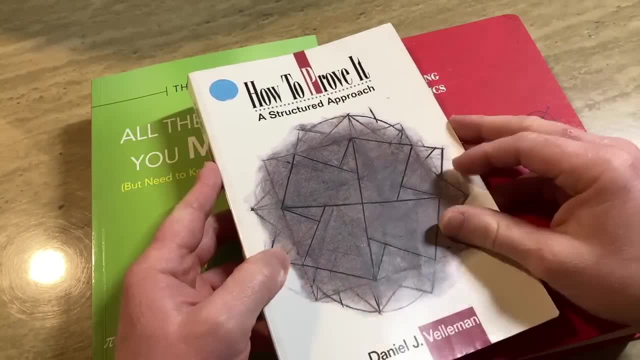 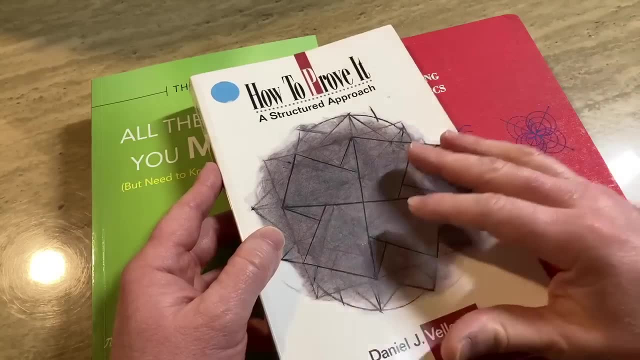 hey, you know, have you looked at the Vellman book? You should check out the Vellman book, And I think it was because I had talked about another proofwriting book. I don't recall which one, But it just seemed like there was a lot of interest in this book. 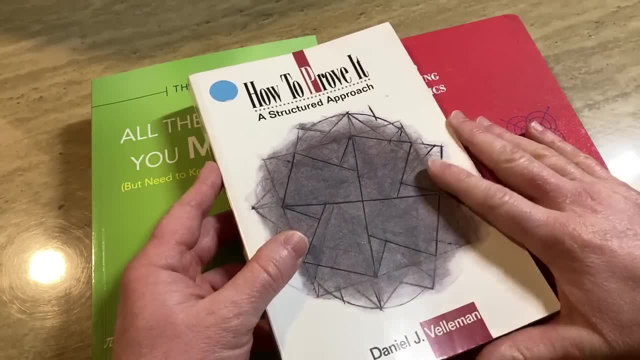 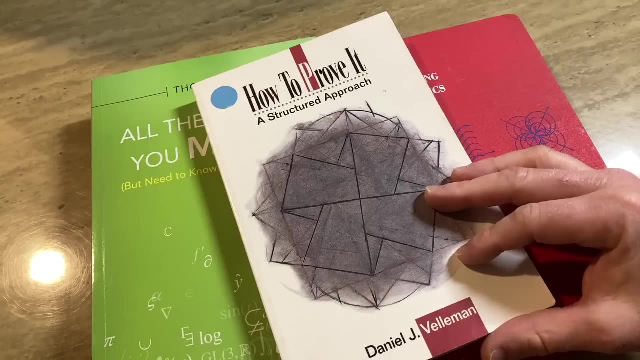 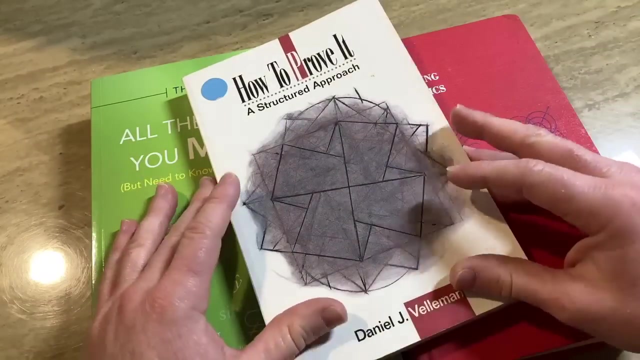 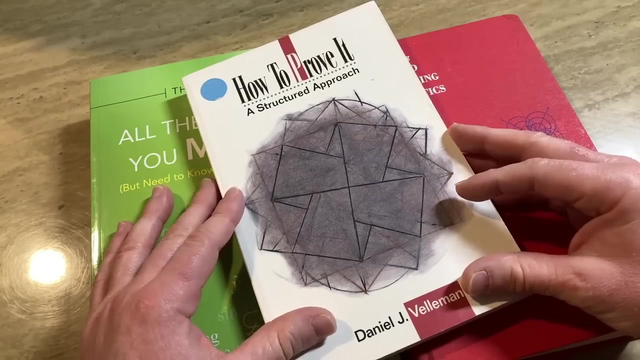 And so I thought, okay, I'll go ahead and buy it. I bought the book And I didn't really want to buy it, I guess because at the time I wasn't really buying a lot of books or I had just bought a bunch And I was like I've already spent too much money. So I bought the book And it wasn't super inexpensive- By the way, I'll leave links to all of these in the description- But it wasn't super expensive either. So I bought it and I thought, oh, another proofwriting book. You know I've seen a lot of these And I was blown away. I feel like Vellman does an exceptional job. 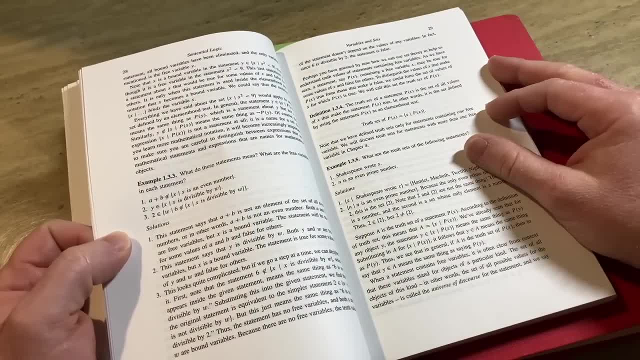 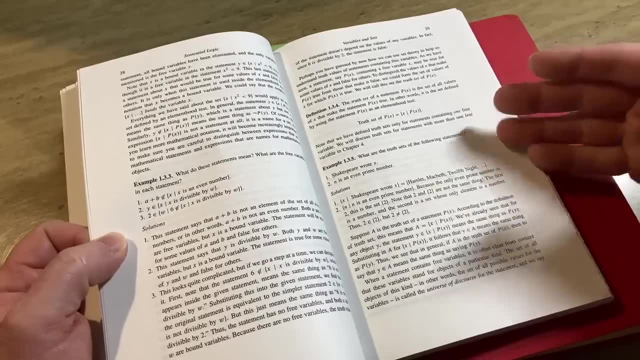 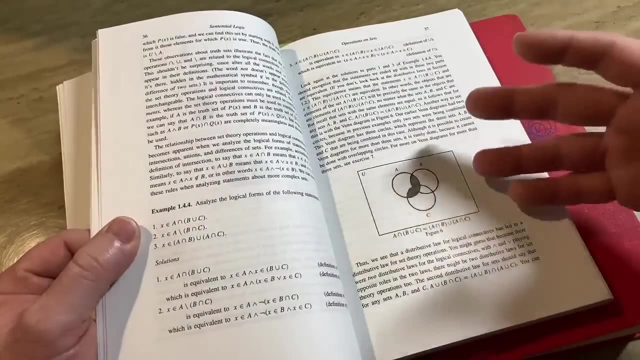 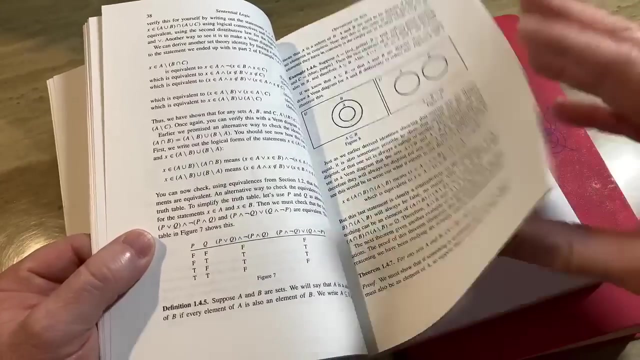 at explaining things or trying to explain things right. Whether or not he explains it depends on whether or not you understand it right. So if you read someone's explanation, if you understand it, then it's a good explanation for you. If you don't understand it, then it's not really a good explanation for you. So, for example, when he talks about vacuous truth, he explains it multiple ways. So what is a vacuous truth? Let me just tell you. Let's just say I say that all, let's see all dragons. 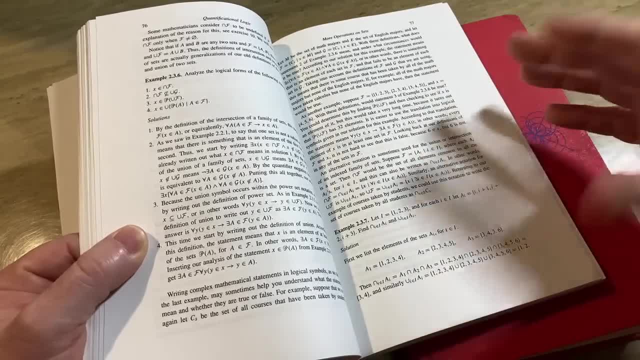 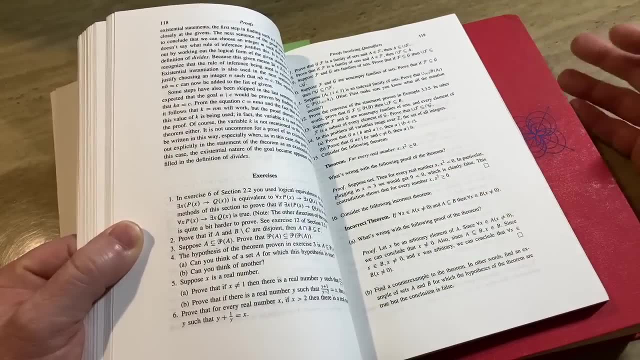 like pepperoni pizza. okay, All dragons like pepperoni pizza. So that's true Mathematically. that's a true statement. okay, in math. In the real world, right? Unfortunately, there are no dragons, Unless, of course- well, I don't know- I was going to say something silly about being a 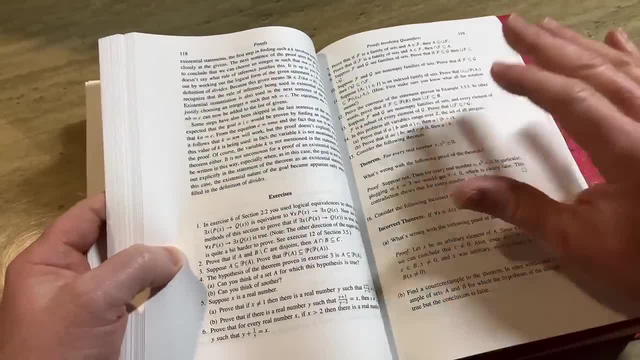 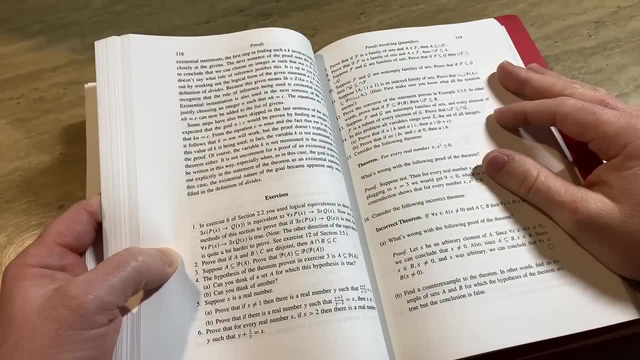 math sorcerer. But let me not, Let's stick to math. So right, So it's true, because there are no dragons. Or if you say you know all people who can fly love hamburgers, right, That's a vacuous. 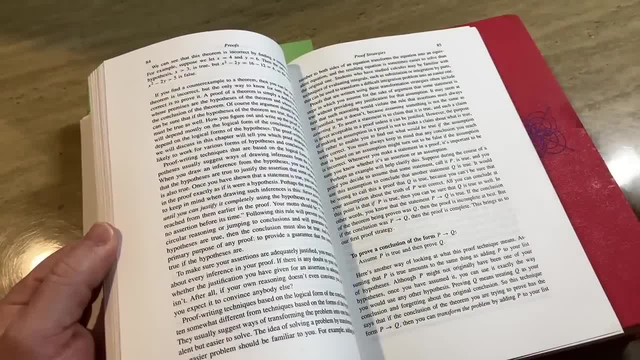 truth because there are no dragons. And if you say you know all people who can fly love hamburgers, there are no people that can fly, right? People don't have wings, They're not birds, They can't fly. So vacuous truths are statements that are true even though they really shouldn't be true. 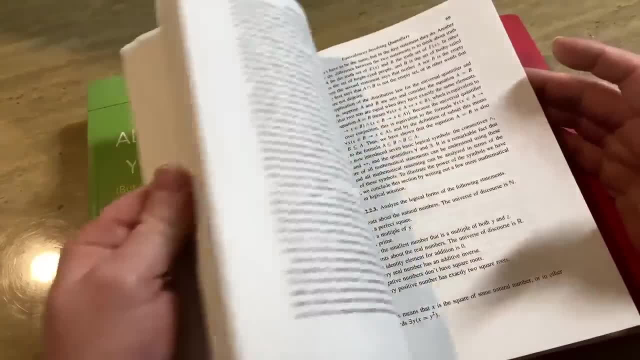 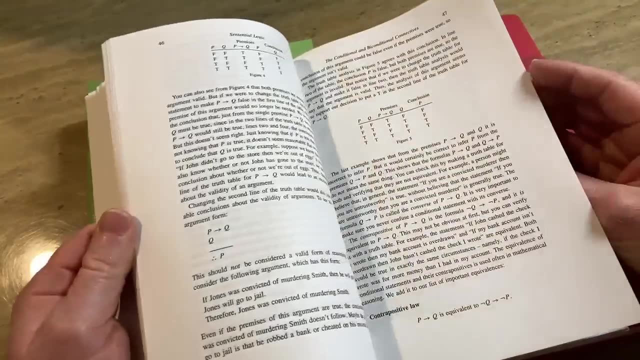 And in the world of mathematics they're true, which is kind of interesting, right? Because you know, a lot of times people think that math is discovered. It is, But at the same time it's created, And that's always a big debate. I think some of it is created and some of it. 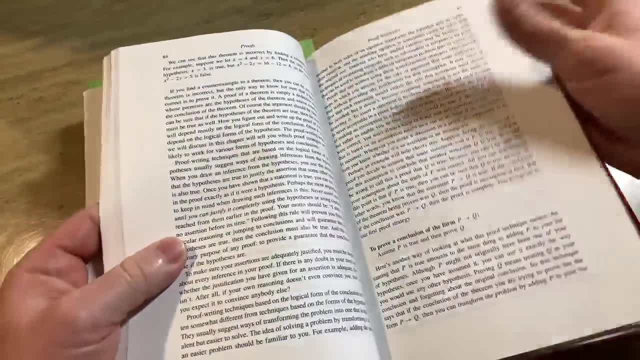 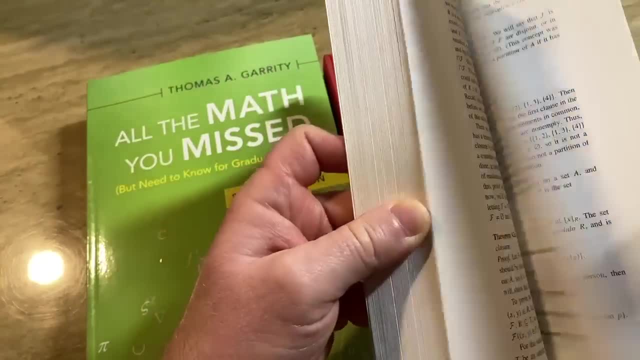 is discovered. It's weird how math shows up in different areas in the world. Let me show you where he talks about the vacuous truth stuff So you can see mathematically why that's the case. So page 68, let's take a look at it. 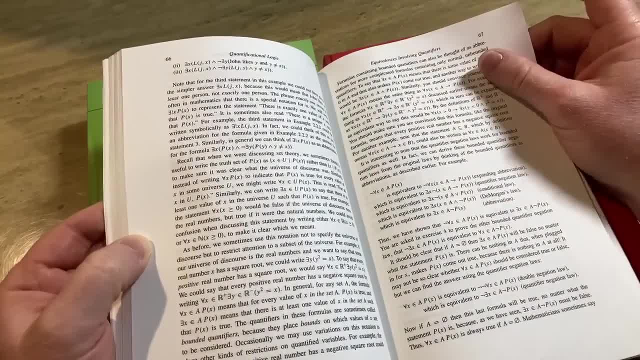 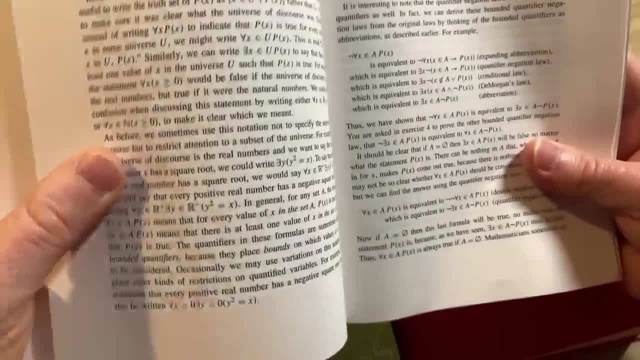 For example, if the kid says I ate all the vegetables on my plate and he has no vegetables on his plate, it's a true statement In the real world. it's false In mathematics it's true. So here he explains. he goes through the explanation of you know why, mathematically. 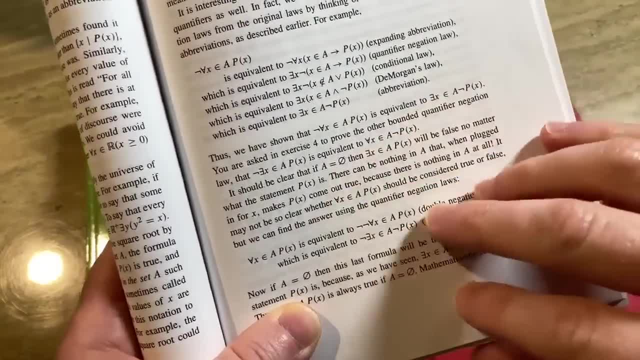 it's true And it has to do. I won't go through it in detail because I want to read all this to you, But basically it's true And it has to do. I won't go through it in detail because I want to. 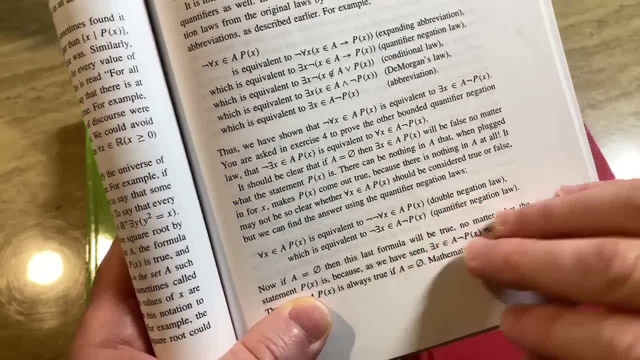 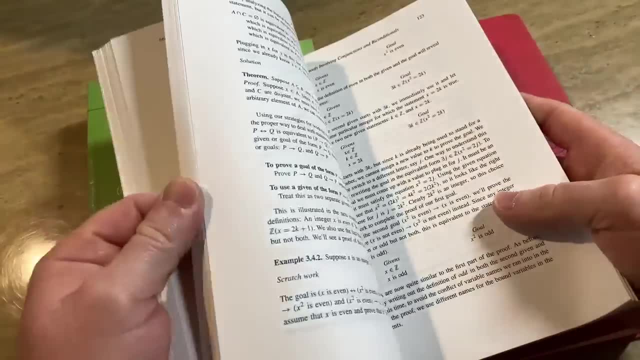 read all this to you, But basically it's true And it has to do- I won't go through it under üchtig. It has to do with logic, with mathematical logic, which is the foundation of mathematics, right Logic, And he takes that approach throughout the entire book. 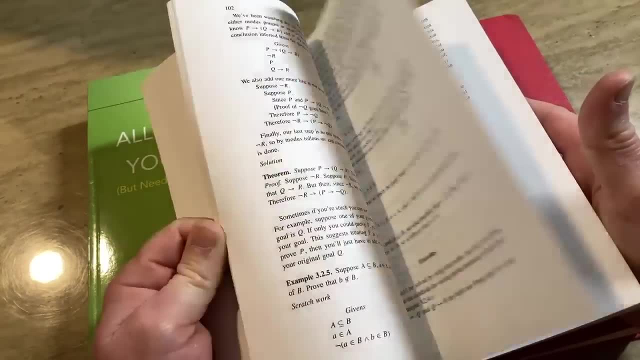 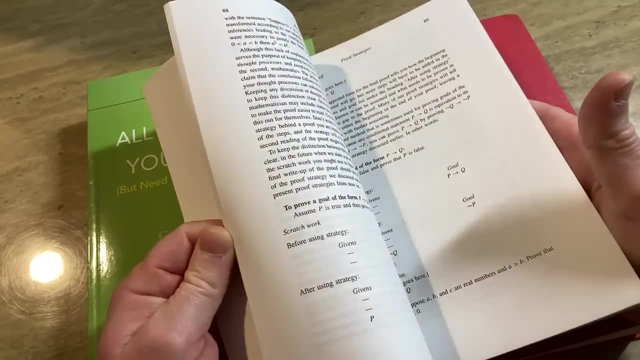 which is super important when you're learning to write proofs. You have to understand logic. You have to know how to negate the definition of. you know uniform continuity or you know convergence of an infinite series. You know you really have to know your stuff, And so 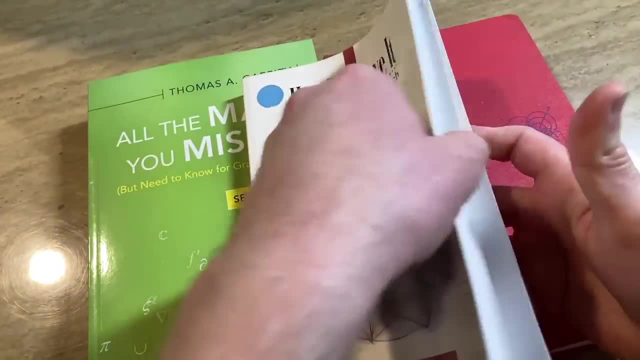 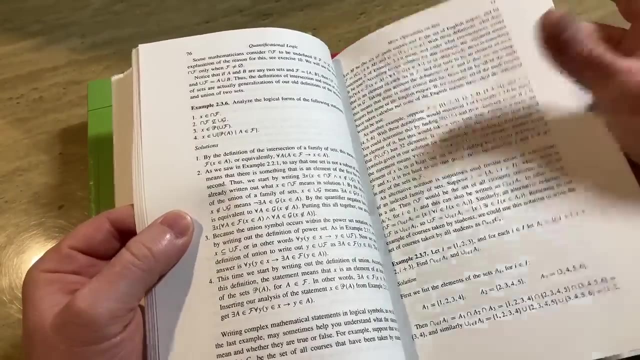 this gives you a really good grounding in mathematical logic. The book has a lot of really good examples so I feel like he does well with the examples. There's good sample proofs. It's a smaller book, It is a soft cover, but it's a nice book for bedtime reading. 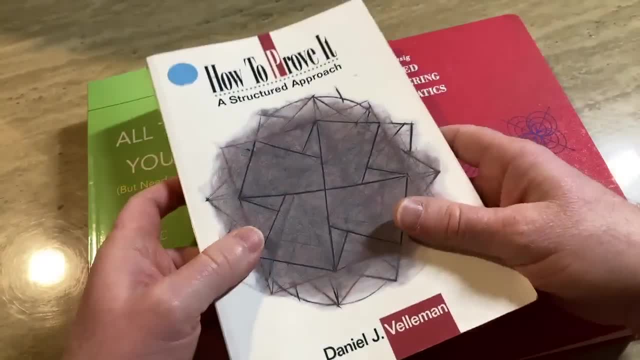 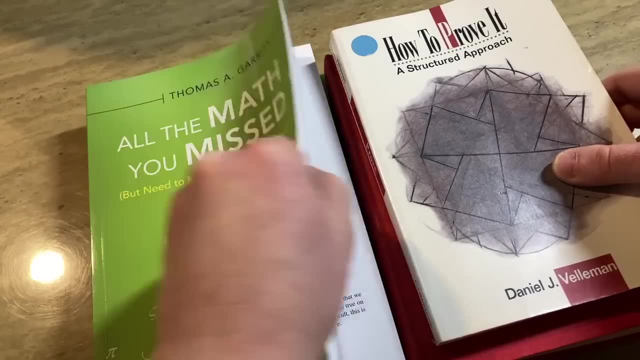 I think this is good for anyone who wants to learn to write proofs, anyone interested in math. This book is easier to read than this one. This one has a lot more math and a lot of- it might seem- more high level. I like this book better. 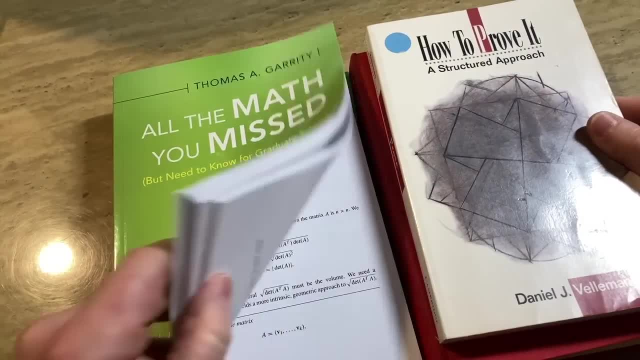 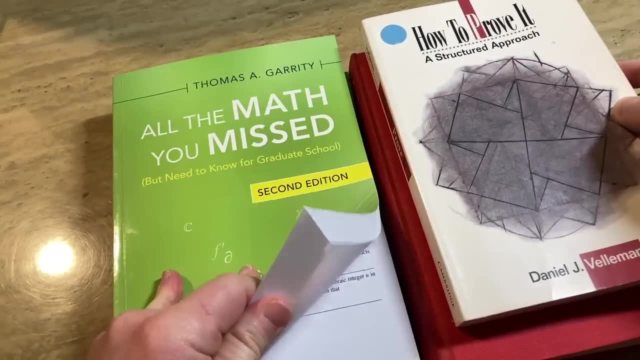 Whoops, moved my camera there. I like this book better because it's more interesting to me, because it has more topics, whereas this- you know, I have a bunch of proof writing books already- This has some interesting stuff that is a little more interesting, but good book for. 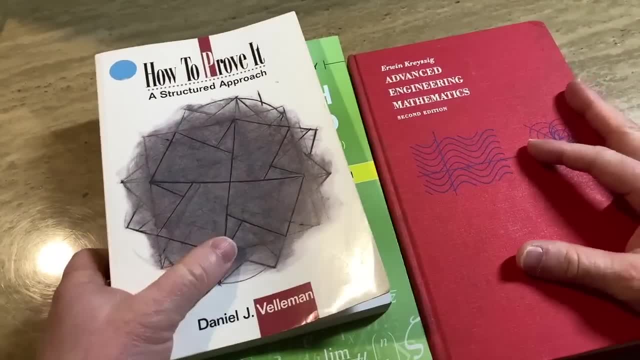 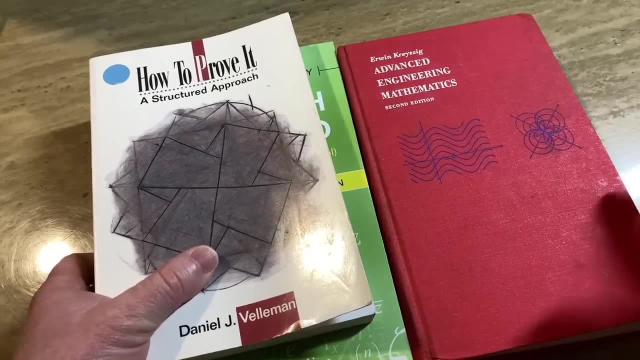 learning to write proofs. This last book which I wanted to show you in this video is the one by Erwin Kreizig, and this is a good book for anyone who likes math or physics or engineering. So it's called, yeah, Advanced Engineering Mathematics. 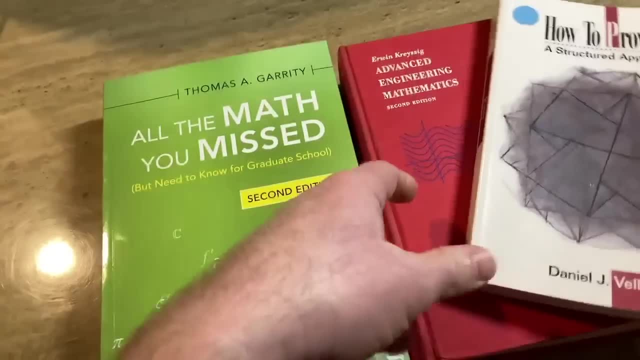 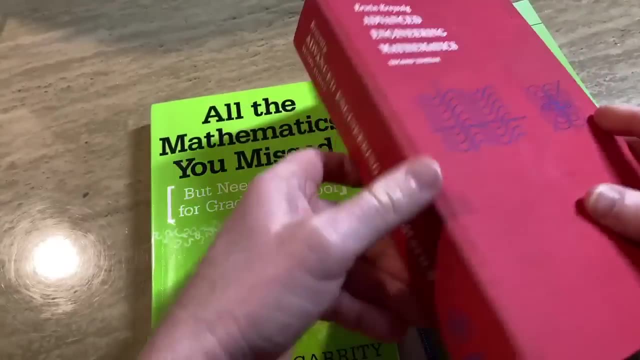 It's got a lot of applied math in it. Let's take a look at it. Just going to pick, The camera hasn't frozen. That's really really good. See if, hopefully, I can make it through this whole video. Look how thick that is. 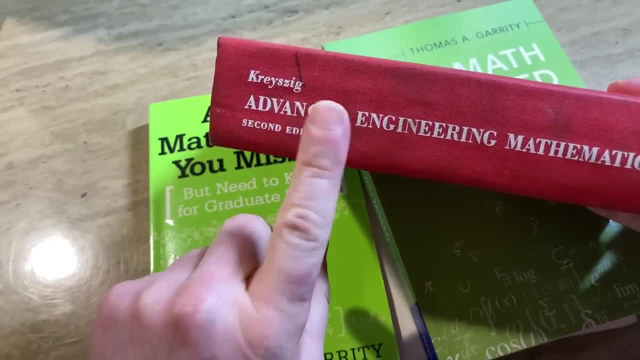 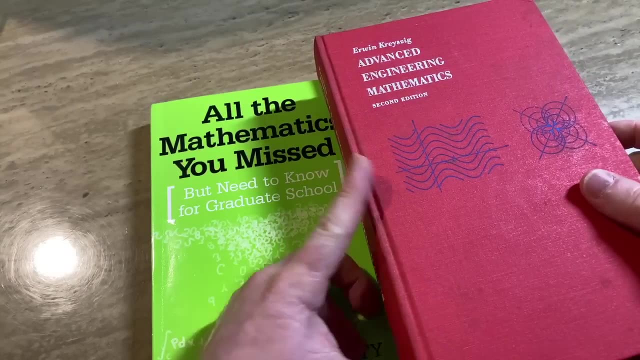 I'll leave links to all of these in the description. This one's more expensive, unfortunately, So this one cost a little bit more. It's a really big book. Kreizig has another really good book on functional analysis, So it's in my opinion his functional analysis book is the easiest functional analysis book. 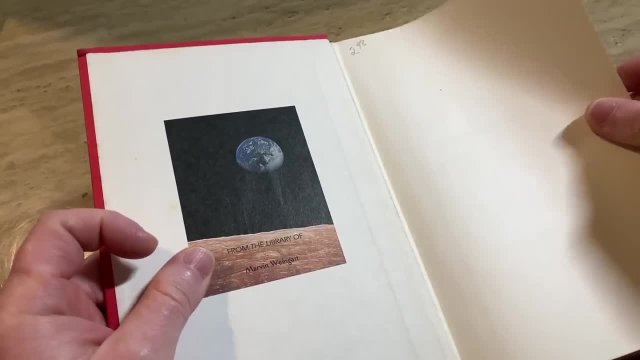 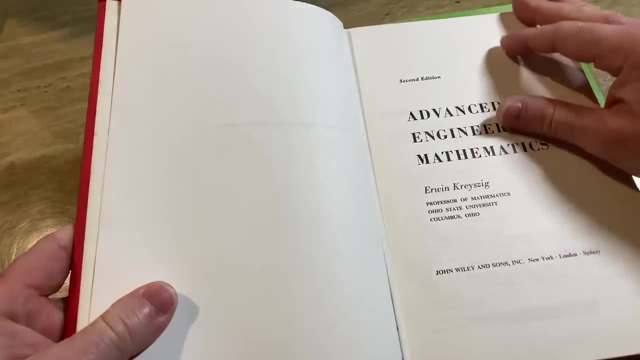 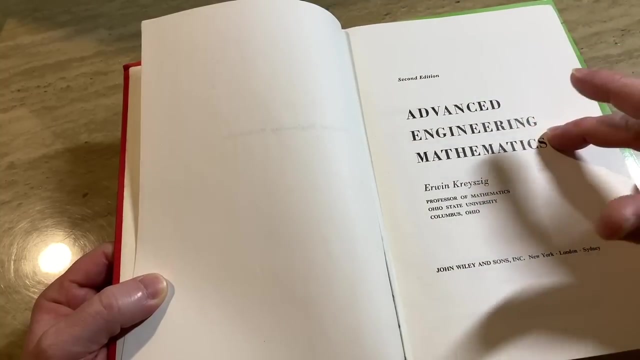 ever written. There's the previous owner And yeah, wow, wow. Advanced Engineering Mathematics: This is the second edition. This is one of those books that other people buy besides math. people like engineering students will buy this book, or like physics people will buy this book. 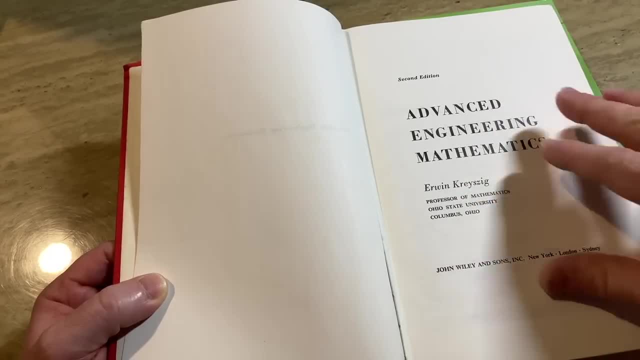 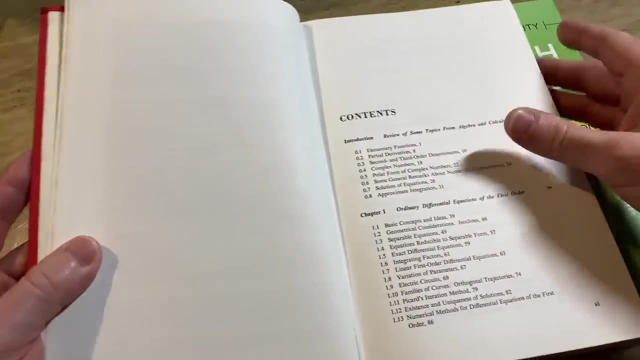 I feel like I knew someone who was taking a course who had this book And let me just show you the topics, because that's really the interesting part about this book. So let's look at the topics. Review of some topics from Algebra and Calculus. 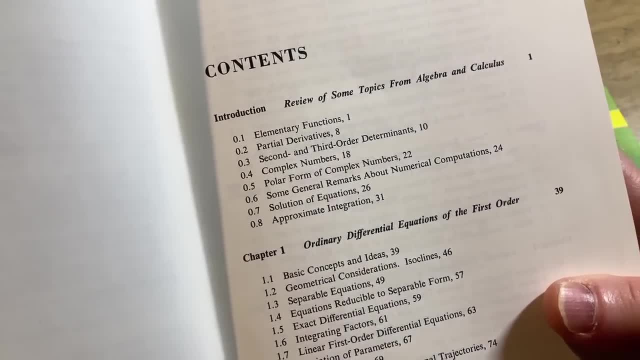 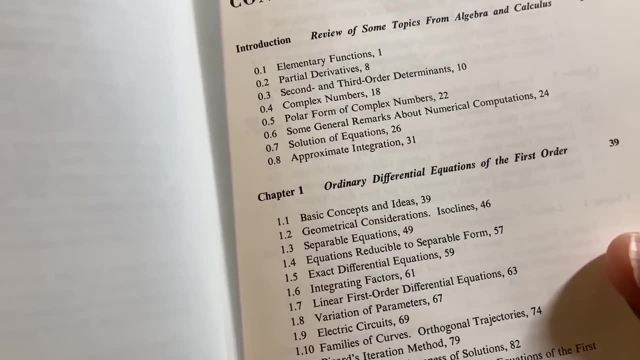 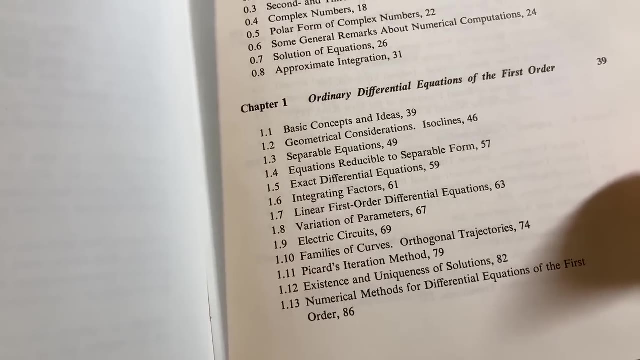 Okay, So look at that: Elementary functions, partial derivatives, second and third order determinants, complex numbers, polar form of complex numbers and then ordinary differential equations of the first order. So if you take a DE class, an undergraduate differential equations class, you learn all. 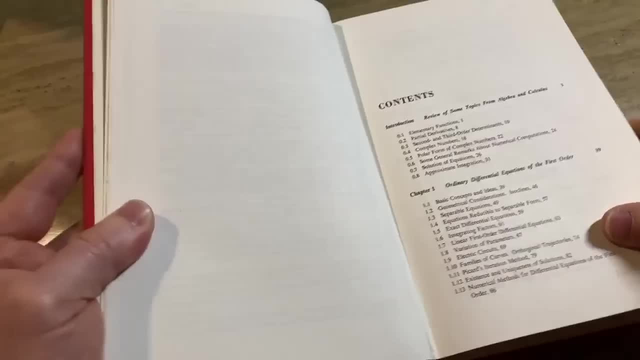 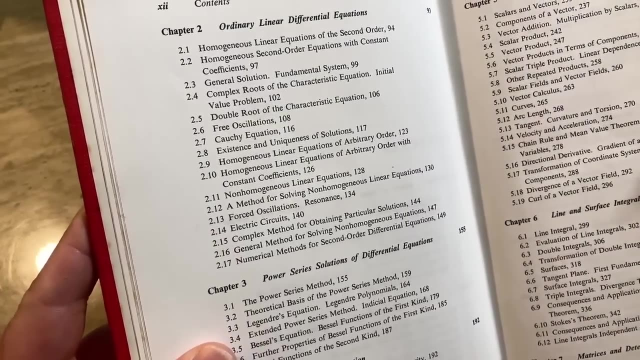 these things. So it covers pretty much the really important stuff in differential equations, right? And then look more differential equations Looks like: okay, higher order stuff. okay, Homogeneous linear equations of the second order, Probably some variation of parameters in there. 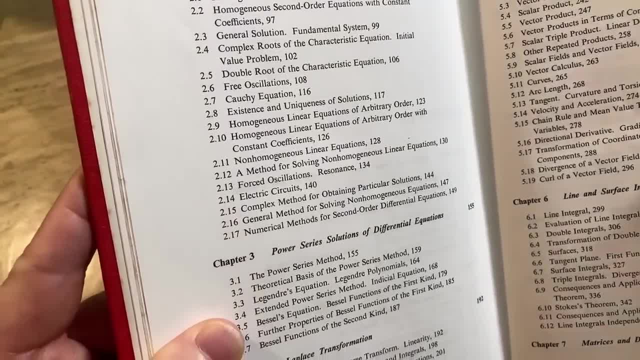 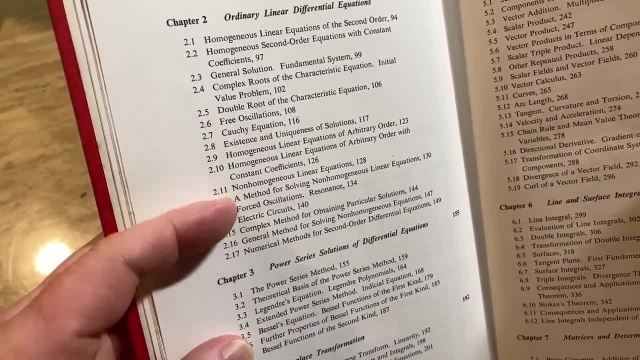 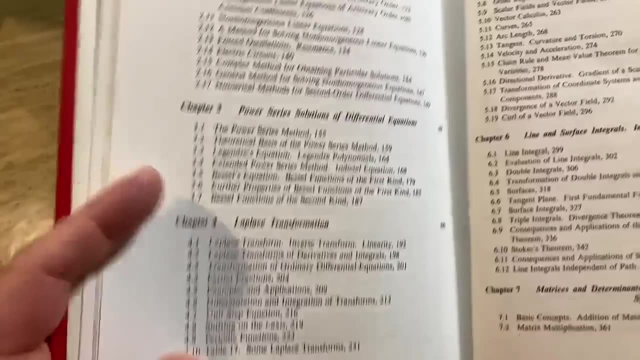 I'm thinking, I don't see it yet. Yeah, I'm sure it's there. Double roots, Okay. Non-homogeneous linear equations- Maybe it's there. Electric circuits, Power series methods, Laplace transforms, Vector analysis. 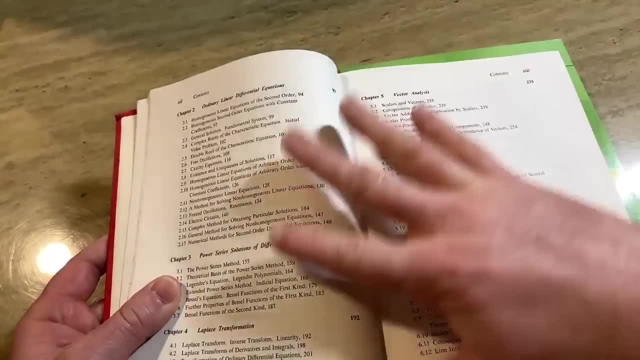 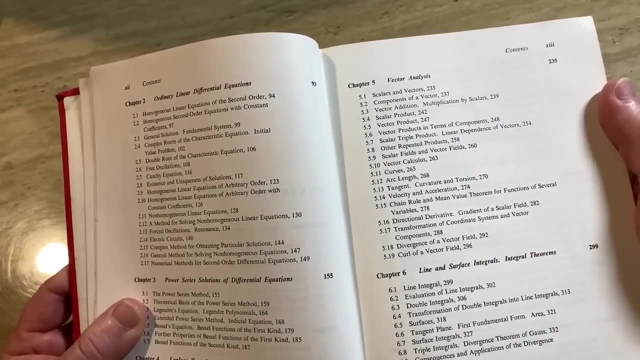 So okay, So you've just gone through and you've learned differential equations with this book. Now you've got vector analysis here, right? So you've got some vector calculus. These are topics that will show up in a Calc 3 class. 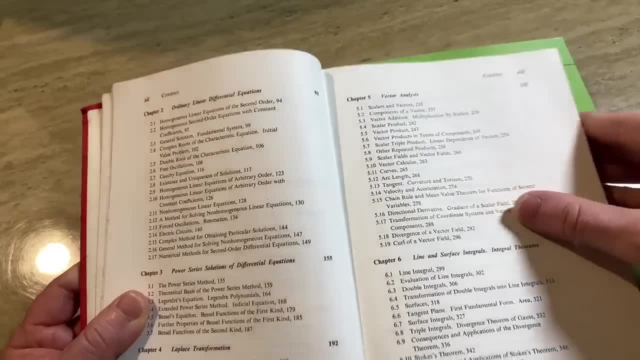 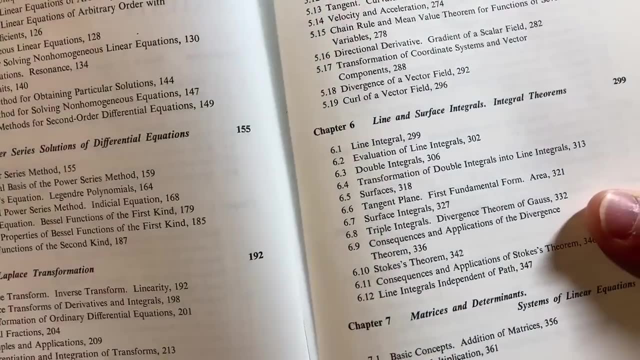 If you ever take Calculus 3, you'll see some of these things. So this will help you for a differential equations class. It'll help you for a Calc 3 class. Here's more Calc 3.. Line integrals, surface integrals, triple integrals, Stokes theorem. 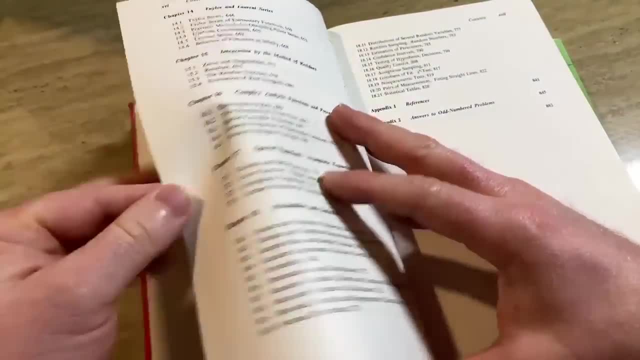 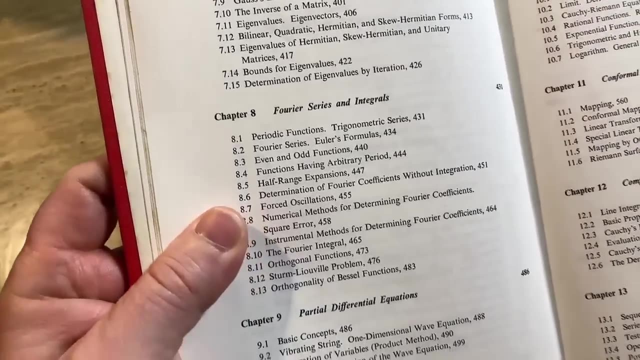 Then you've got some matrices and determinants. You've got linear algebra in this book. I mean completely ridiculous, Just insane. What a great book. Yeah, Look at that. And then Fourier series and integrals- Something you might see in an applied math class or in a partial differential equations. 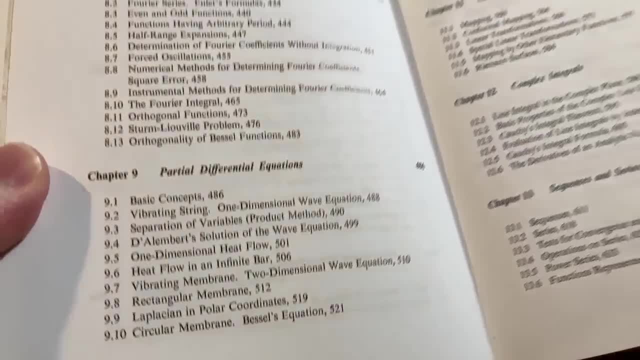 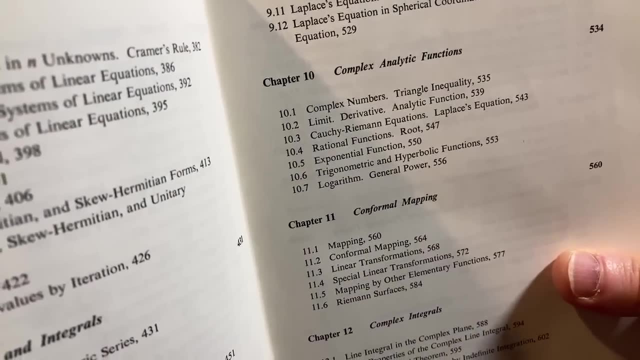 class, And then partial differential equations right after that. Well placed, Mr Kreizig, What a legendary book. Then complex analytic functions. So if you took a course on complex analysis or complex variables, you would learn these things. So I mean just tons of stuff. 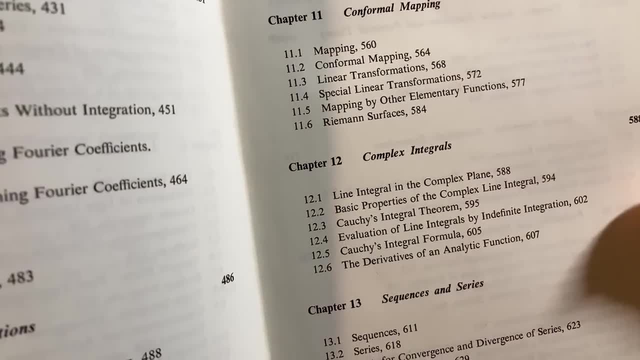 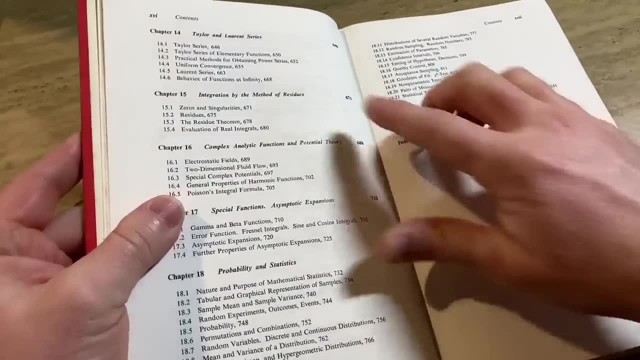 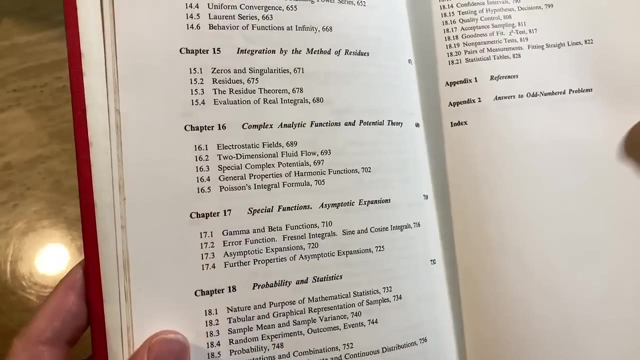 Conformal mapping, Complex integrals- That's also something you study In complex variables, Sequences and series. That's Calc 2 stuff, Taylor and Laurent series. Integration by method of residue- It's more complex variables, Complex analytic functions and potential theory. 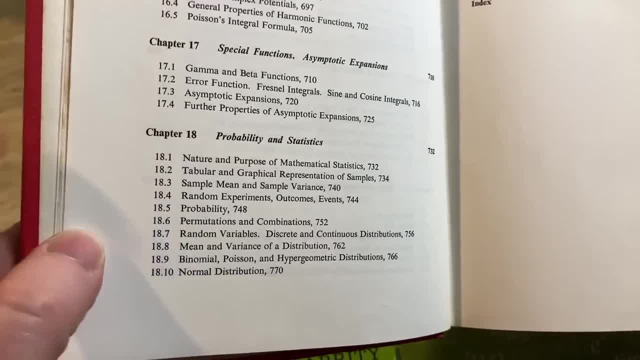 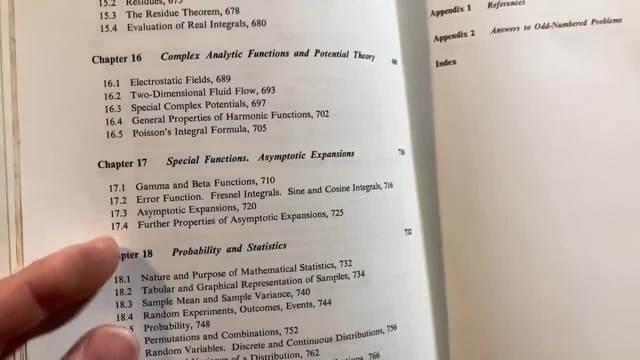 Special functions, Gamma and beta, Then probability and statistics. Right, He's like: you know what? Let's throw in some probability and statistics in chapter 18, just for good measure. Let's just throw some in there because we're awesome. 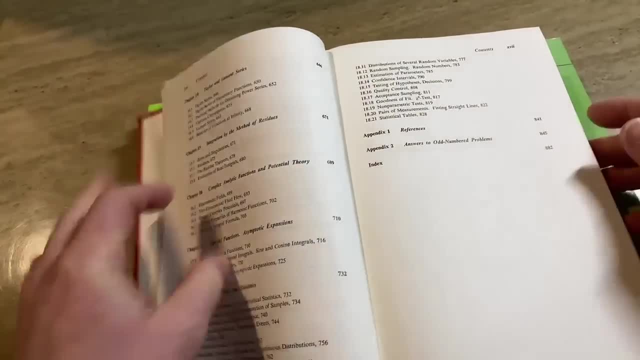 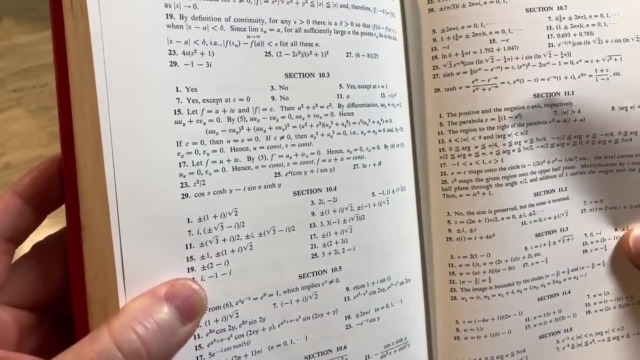 I mean insane. It has answers. Right, It actually has answers to the odd-numbered problems. Let's just take a look at that. I actually have two copies of this book. Yeah, pretty cool, Pretty cool book. I just got to give it a whiff. 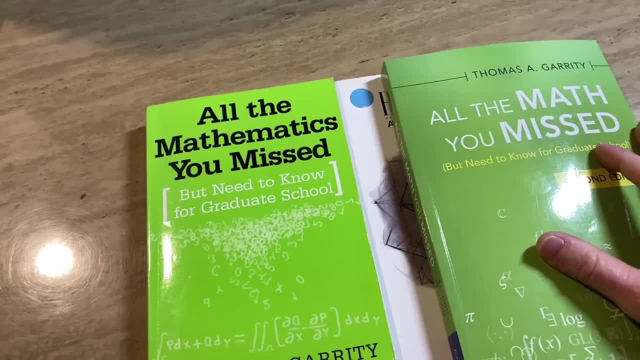 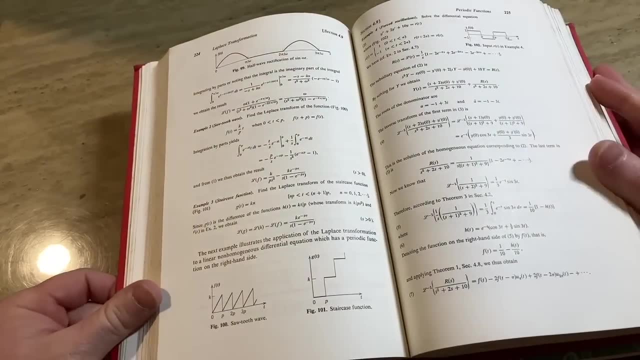 I'm just going to move it out of the camera here because I got to smell it Just. Oh, it smells so good. What an amazing book. So the contents are awesome. The price is not It's expensive, But honestly it's Kreizig. 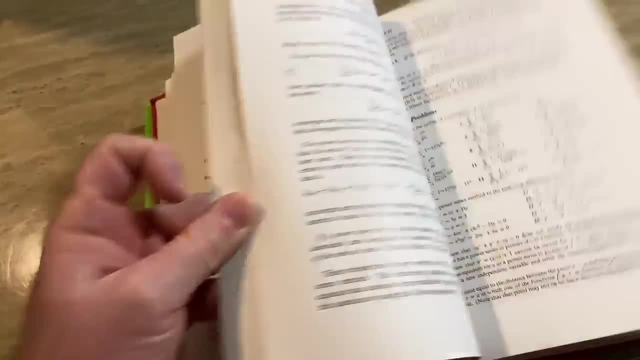 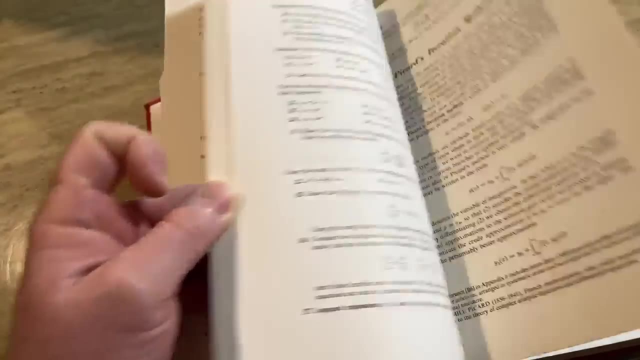 I mean, this book has so much math. I always think that math books are priceless. I really do, because I collect them. So, as a collector of things, that's just how I am. But yeah, I mean very, very clean layout. 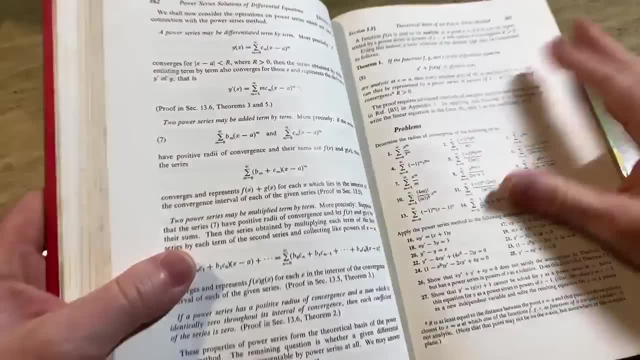 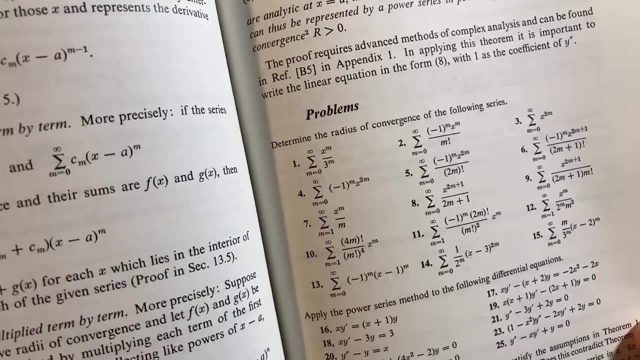 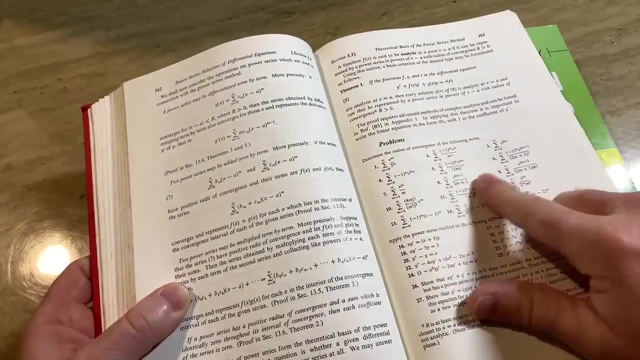 Let's just open it to a random page. Theoretical basis of the power series method. Okay, This is cool. Oh, this is cool. This is something you might have seen before: Determine the radius of convergence of the following series. So if you're wondering why it's called the radius of convergence, so here, when you find 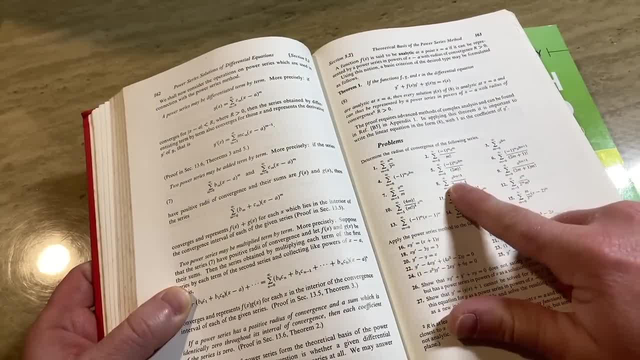 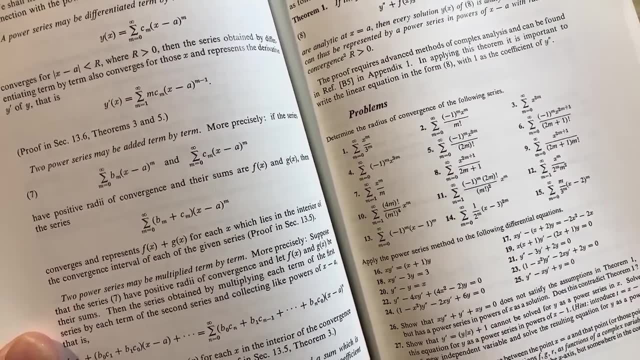 the interval of convergence, If you were to find that for these series it's an interval, right? So it's a subset of the real line, right, Like one to infinity or zero to infinity. So why is there a radius, or one to three? 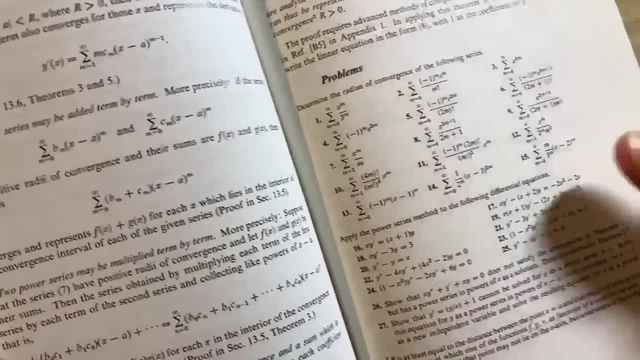 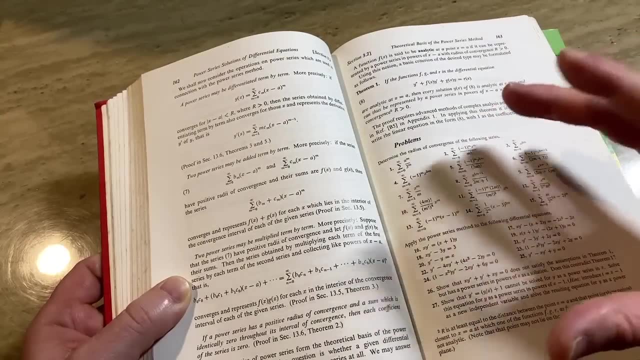 So why is it called radius? It's because if these were complex variables, like if X was a complex number, instead of an interval it would be like a circle, It would be a disk And the radius is the radius of the circle. 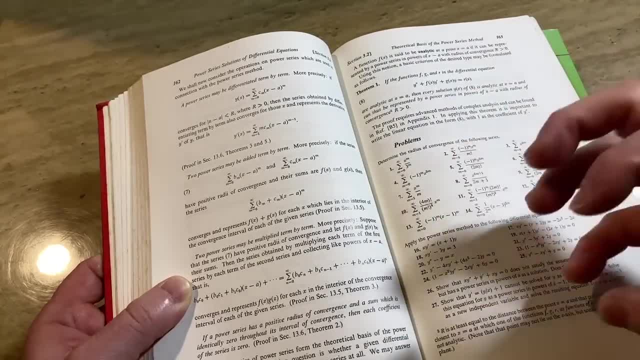 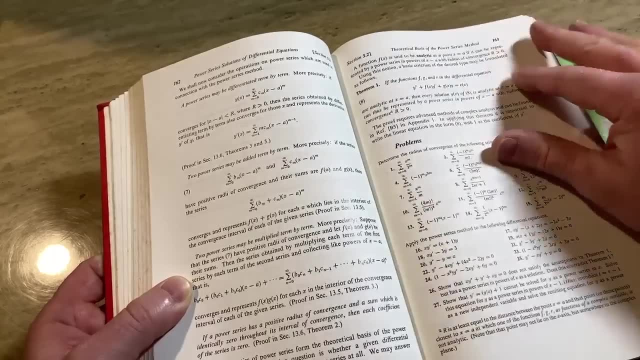 Okay, So you know a disk is. you have an open disk or a closed disk. An open disk is basically a circle with dots and then everything inside is shaded. So there's an actual radius there and that's why it's called radius. 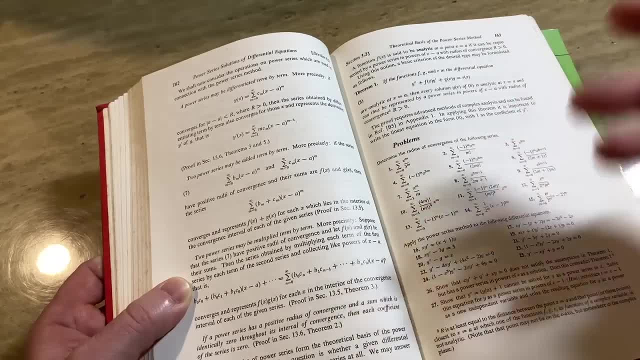 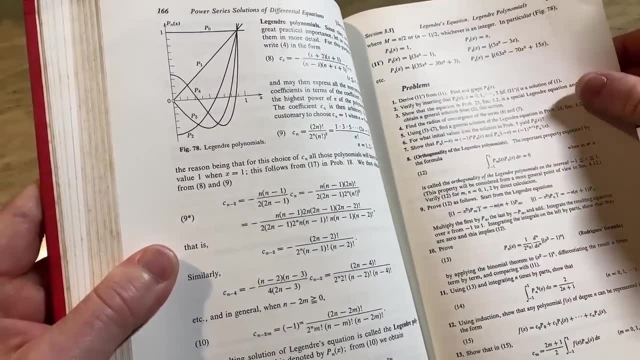 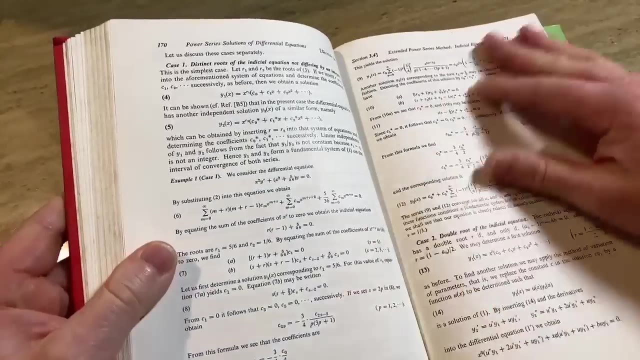 But when you study calculus it's not an actual radius, but they still call it radius. So it's because of complex numbers, but kind of random. These problems are really long. when you start solving differential equations with power series, They can get pretty insane. 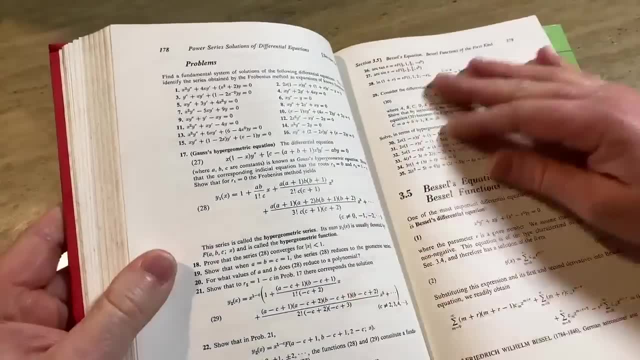 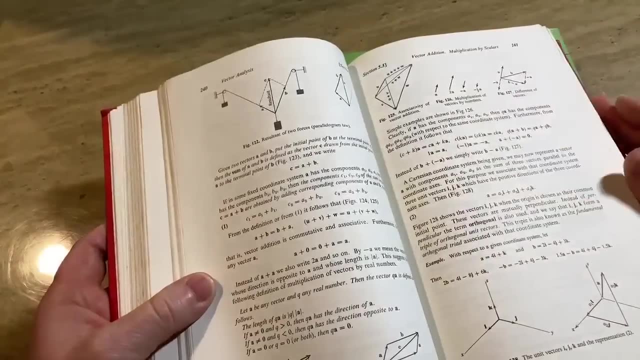 So yeah, Pretty cool book. Yeah, I just like it a lot because it has so much math and you know what you can do with this. you know how do you use this book. You can use it as a reference, but you can also use it another way, right? 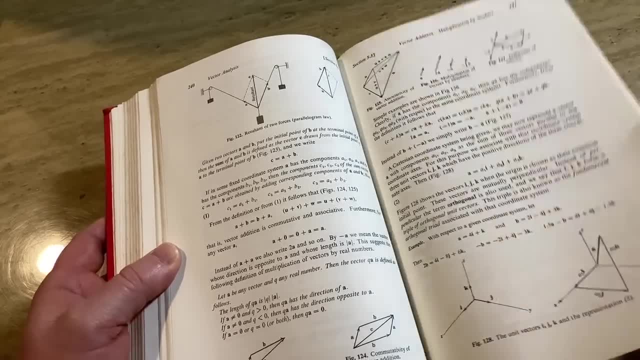 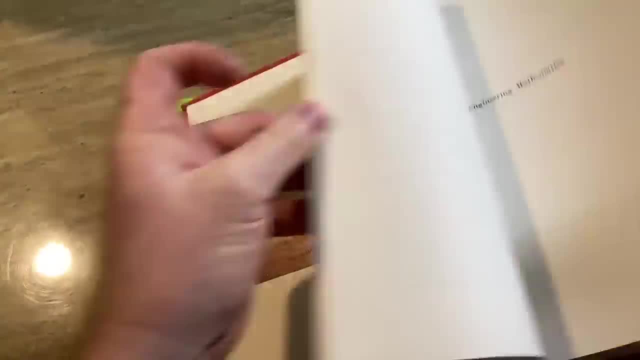 Like, let's say it's raining outside or you just, you just want to be away from people, or you just want to like study alone. You can take this book and you can do the following. I'll just show you Like you can open it up and say: Hey, you know. 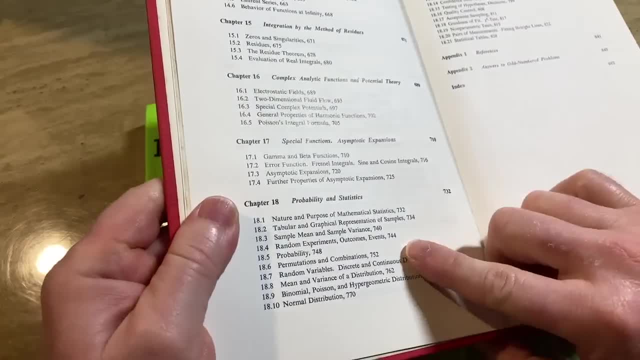 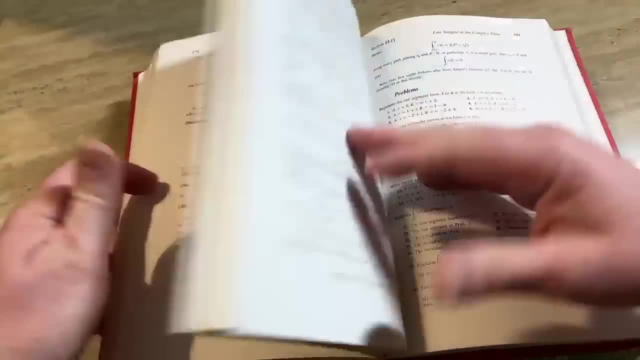 I really don't know that much about. you know, um, probability, page 7 48.. Let's go to page 7 48 and let's take a look at that, Cause I took a stats course but, like you know, we use some software. we really didn't. 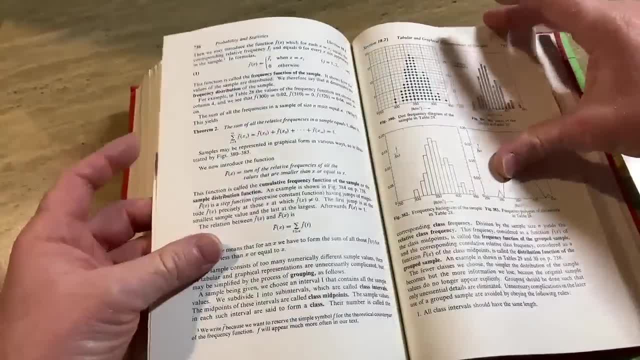 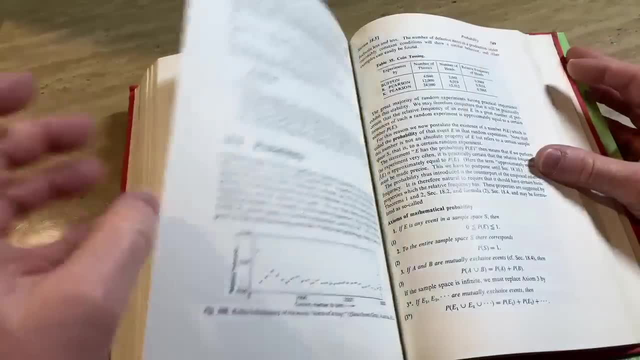 learn much, and that that's. you might've learned the concepts, but maybe you didn't learn how to do it by hand. Right, You say, Hey, let's go to probability. The concepts actually are harder. I think the conceptual stuff and statistics is is really tough. but here it talks about. 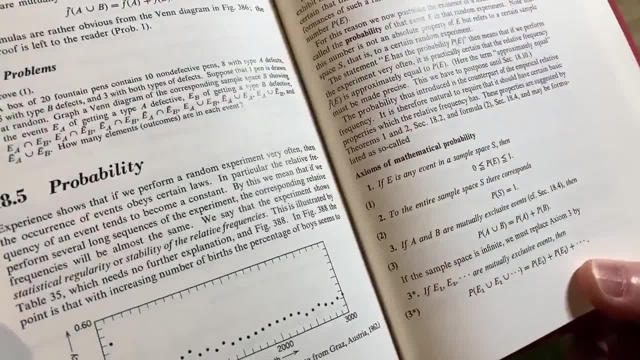 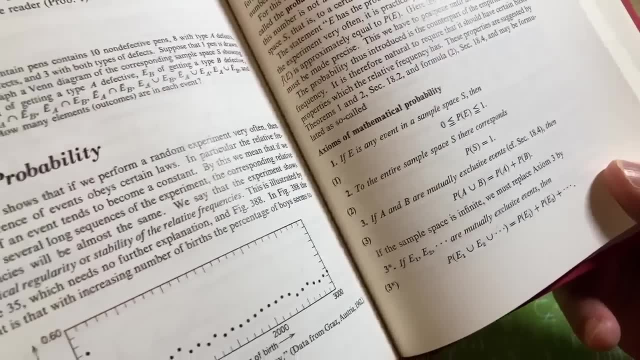 probability, right. And then it talks here. Here they give you the axioms, the axioms of mathematical probability, right. So you study this in college If you take a course on probability. I took a course called statistical theory and it. 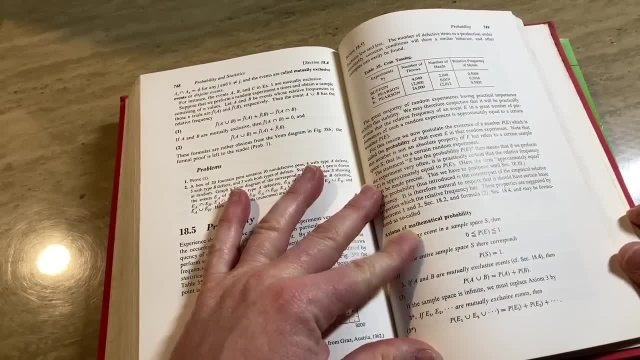 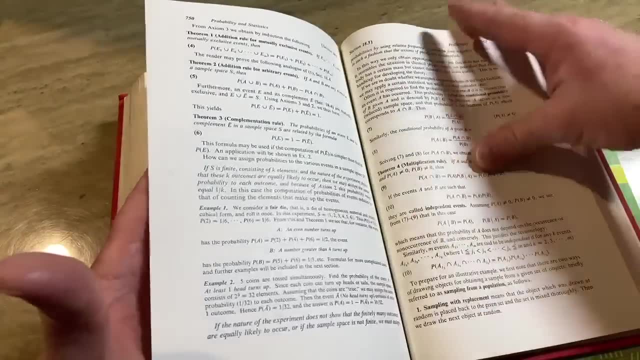 was extremely hard. The prereq was like the full calculus sequence and a proof writing course, I think, And it was so hard And we did stuff like this. We had to do proofs very, very tough when you're learning, So this book would help you. 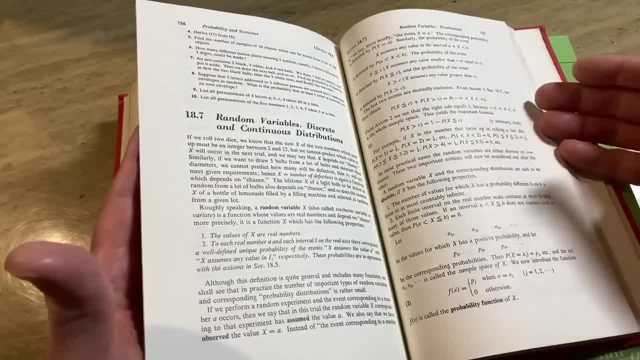 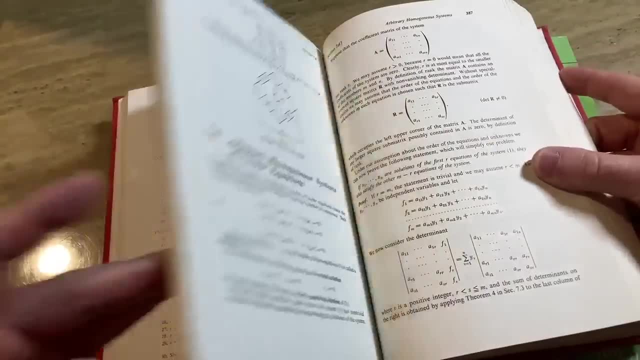 If you took a course like that, It's like that as well. So differential equations, mathematical statistics and probability, complex variables. it's got a lot of multivariable calculus, a lot of stuff with series, incredible books. So this is a book that's good for anyone who wants a solid math book. 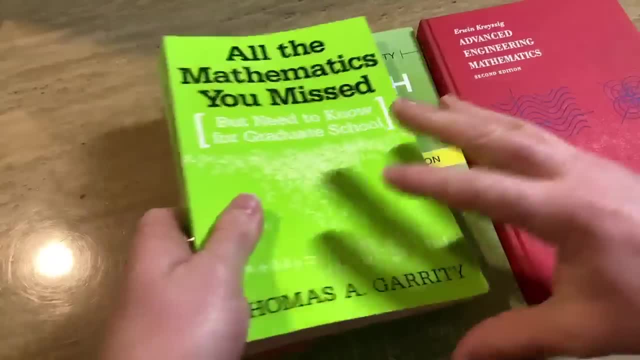 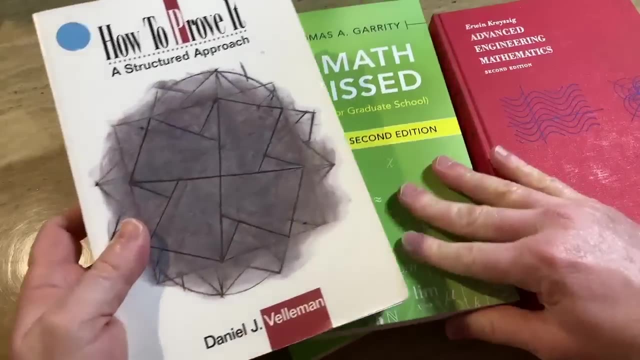 Like this. this book has more material than the other ones that I've shown you, So let me just show you the other books one more time. So this is the good, a good one for proof writing. I'm totally recommended for proof. 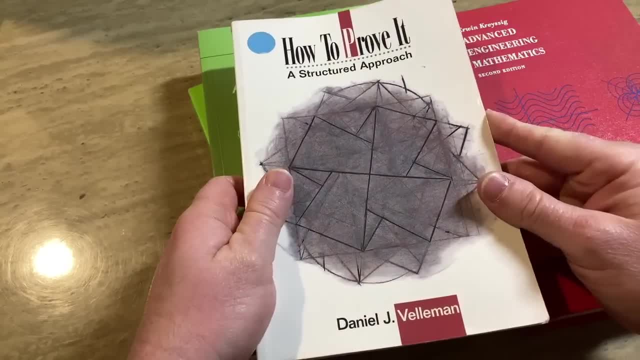 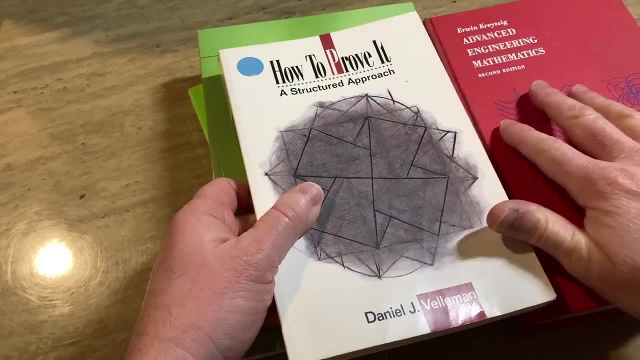 If you want to learn how to write proofs. that's important. You need to know how to write proofs before you jump into higher level math. Like a lot of the math in the Kreisig book is going to require proof writing. Likewise, a lot of the math in this book is going to require proof writing. 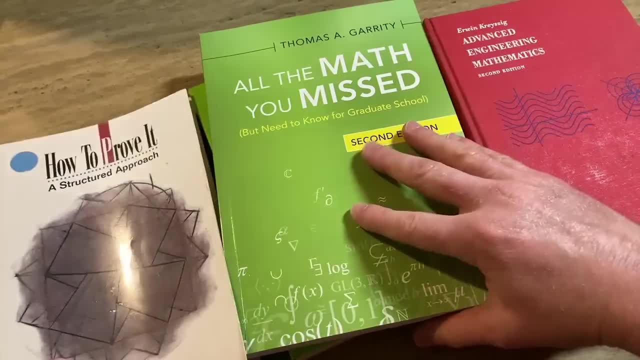 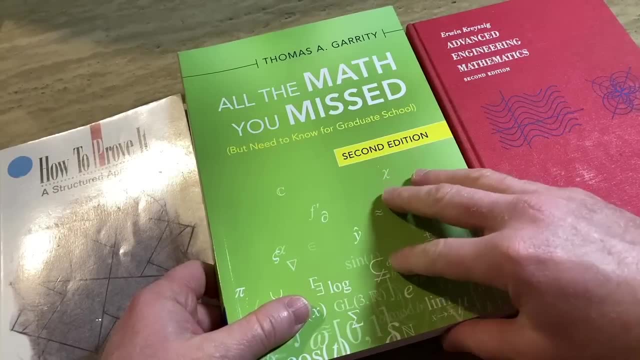 So in some sense this is the most elementary of the three. This book just gives you an overview of various topics in mathematics, which is really cool. There's more topics in this book than in this book And he does do some math and you know there's there's some serious mathematics in this book. 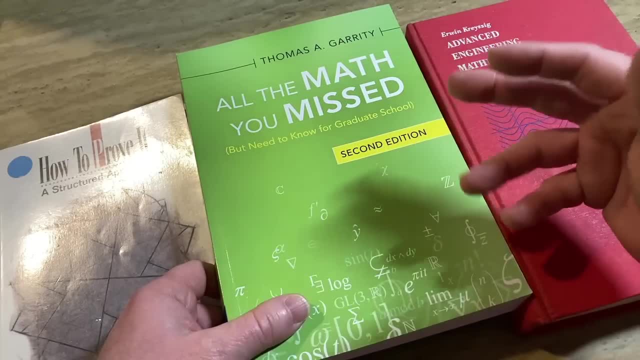 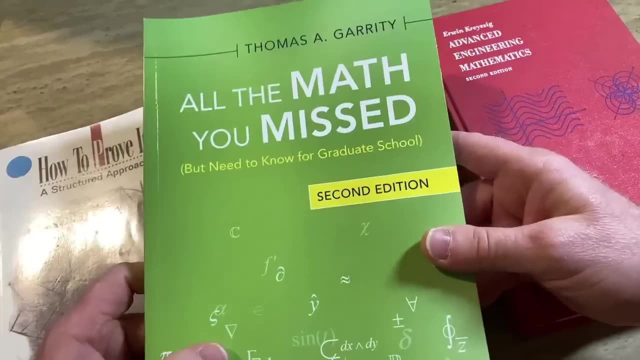 uh, but It gives you an overview And, honestly, that's quite challenging to do that, So I think it's really impressive that you know Thomas Garrity, uh, did that. So this is. this book is going to live on forever. 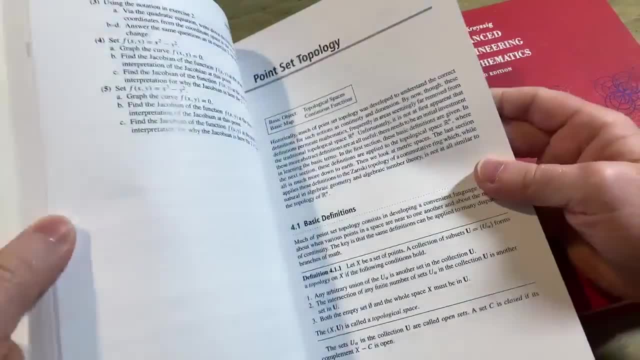 It really is. I think years from now people will be looking at this book and be like: oh yeah, the Garrity book. I mean, I just feel so lucky I was able to, like you know, make a video with him and stuff. 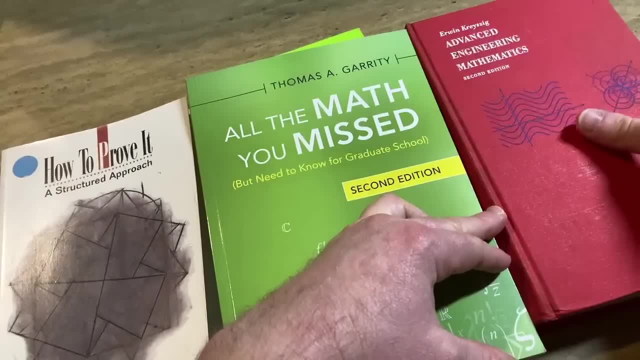 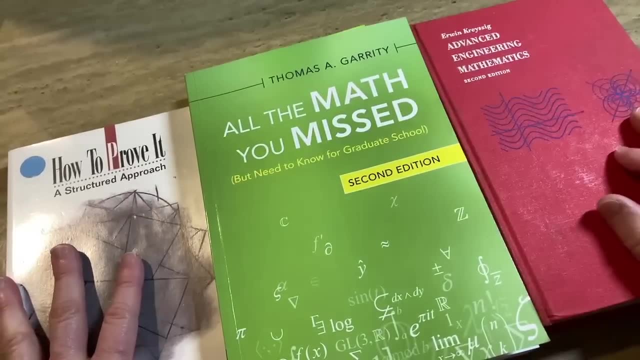 And this book is legendary already. This book has been around for a long time and it covers way more math. Um, just a good reference. A lot of physics people are into this book. anyways, the video is getting a little bit long right. 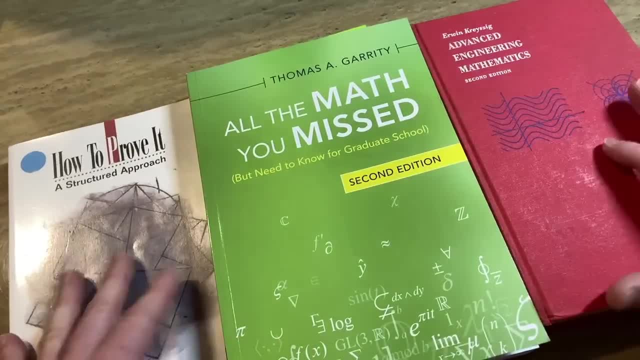 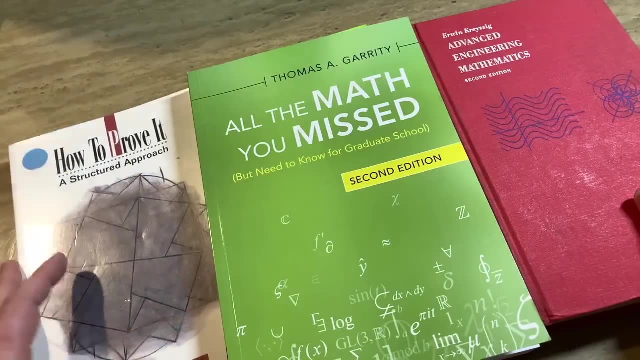 18 minutes. Now I can actually see the time because of my recording setup, but I just wanted to show you math books that I think are for everyone And hopefully- uh, I post this video and it doesn't freeze before I end the video. 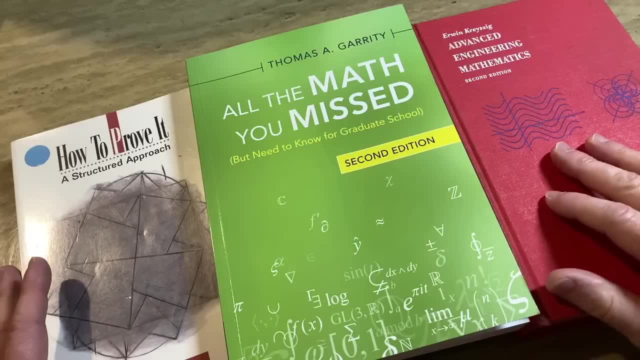 If you enjoyed this video, let me know like: did you like this format? Did you do you like the other format? Um, I think the sound quality is better in this video Cause I'm using my like my stream. 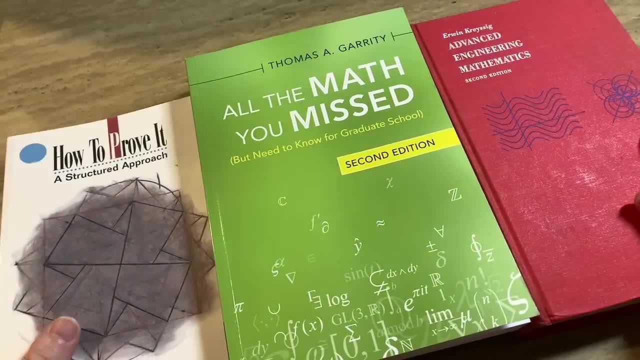 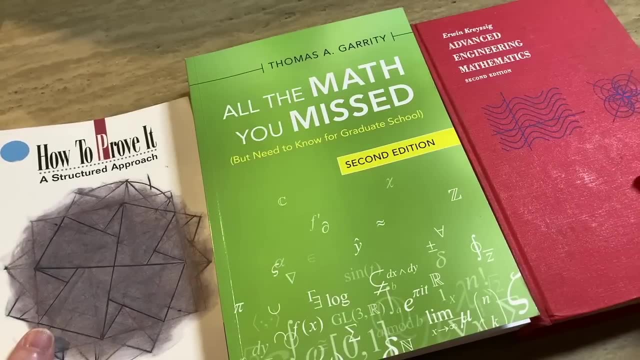 I'm using my like my stream. I'm using my like my streaming setup, which randomly freezes. So hopefully, uh, hopefully- you've enjoyed this video and hopefully you've learned about some- you know, some- really cool books. All of them are awesome. 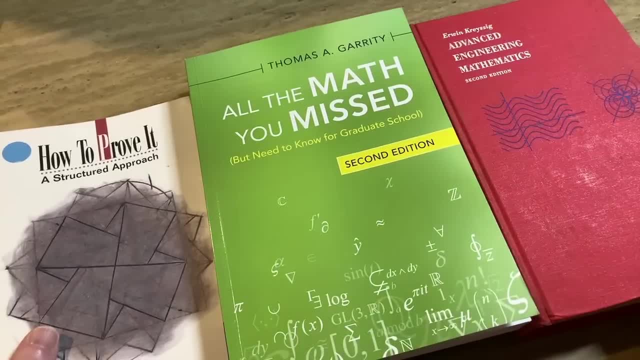 That's why I have them. It's funny, I have two copies of this one and two copies of this one. until next time, Good luck and take care.